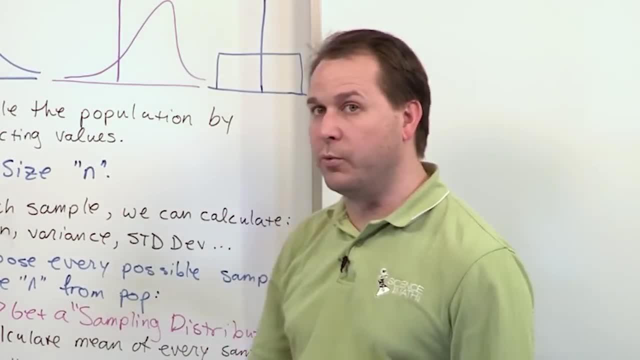 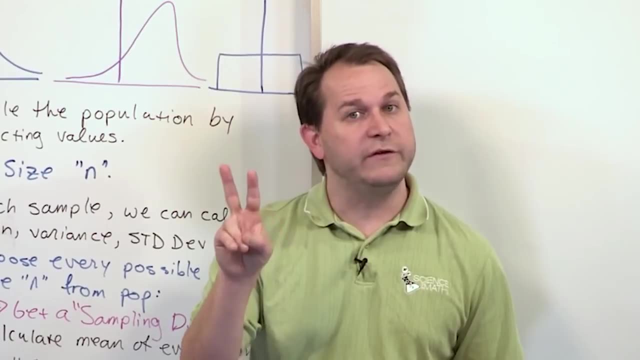 Limit Theorem here, the continuation here. It's why I've left everything on the board, so that we can then learn. So, as we go through the Central Limit Theorem, remember two things. okay, two things, only two. Number one: remember that the Central Limit Theorem is not hard to understand, but 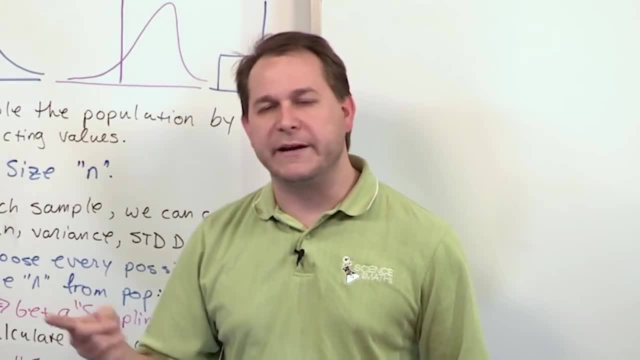 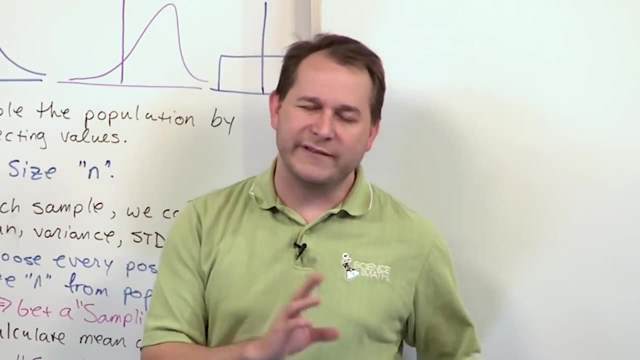 you have to let me get through the whole spiel before you understand it, and probably a few problems too, before we really understand it. Number two: the Central Limit Theorem is very, very, very useful. all right, You don't see that in the beginning, but when we start working? 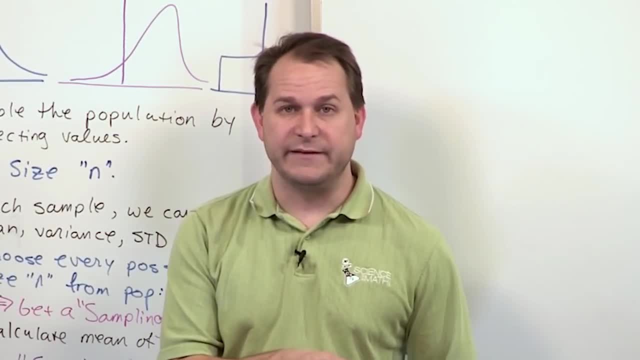 the problems, you'll understand how useful it is to actually have this thing laid out before you. So I'm not going to prove it, we're just going to talk about it. So for the Central Limit Theorem, I'll just go ahead and write this down: it's called: 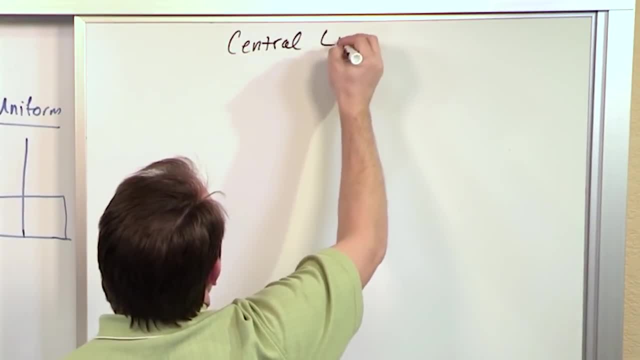 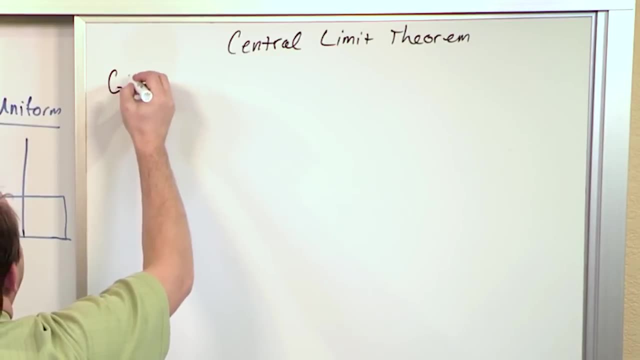 the Central Limit Theorem. all right, And when we're studying this, guys, we have to make some assumptions. So I'm going to say, given this is what you're actually given, when we're talking about, We're given a population, which is what we're trying to study usually. 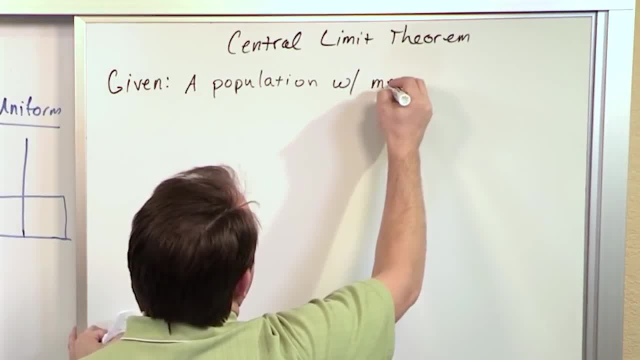 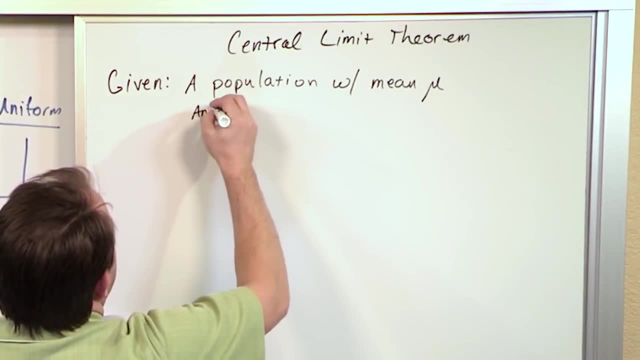 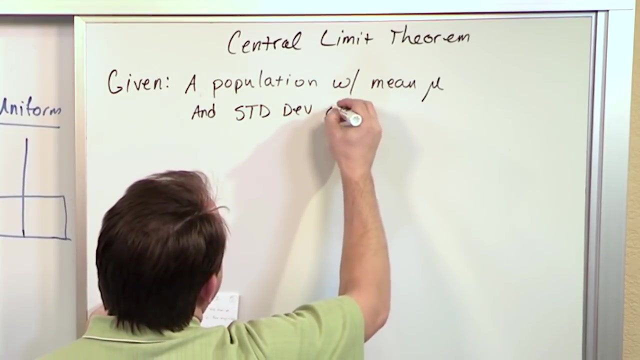 and it has a mean, A mean of mu. remember the symbol: mu, that's the mean of the population, and standard deviation: that's what I usually write down when I say standard deviation. lowercase sigma. that's what the symbol is. We've studied these things before in previous parts of mastering statistics. 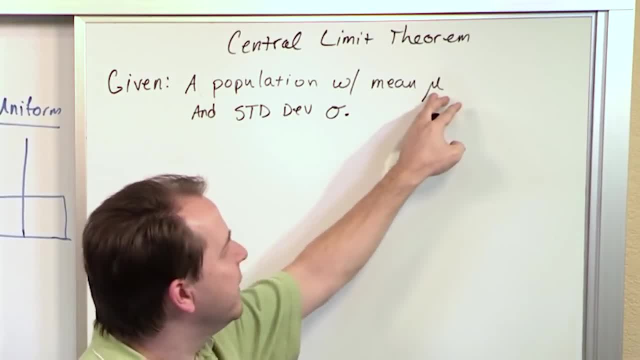 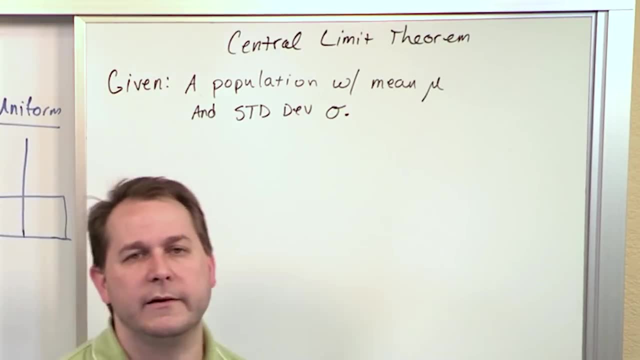 but just reminding you, when we talk about the mean of a population, we're using the symbol mu, like that's a lowercase mu, and when we're talking about the standard deviation, that's a lowercase sigma. that's what a lowercase sigma looks like. If you have no idea what 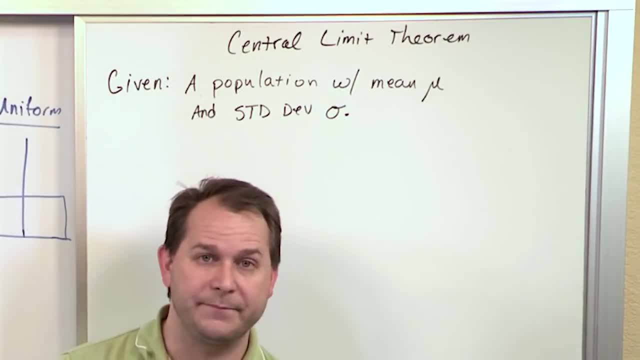 a mean or a standard deviation is at all, then you need to stop and go back to mastering statistics. previous lessons- We study that stuff- make it crystal clear. you need to know what the mean is and what the standard deviation is. But anyway, these properties. 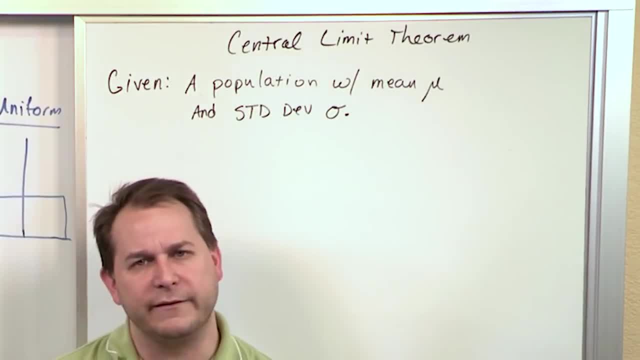 these two properties here are related to the population. So, for instance, if my population is all North American male males, let's say all North American males, that's the large people. I can't study them all directly, But we know that if I'm studying their height, then if 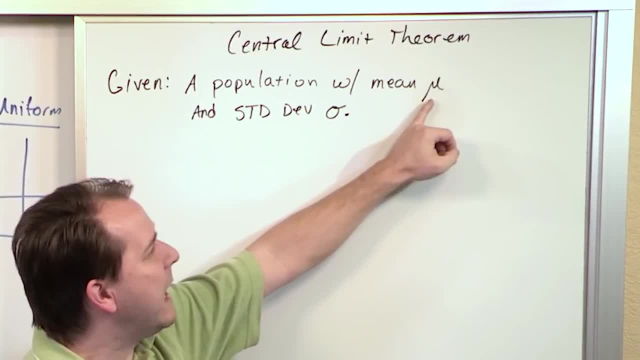 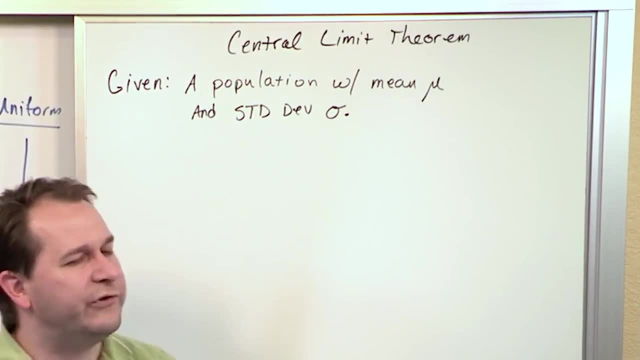 I study all North American males. they will all have an average height or a mean height. we'll call that mu. Maybe the mean height is like five feet eight inches or something, And there will be a standard deviation, which is how spread about that data is about the. 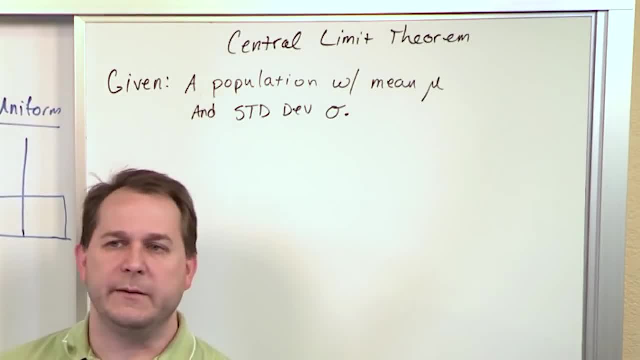 mean. So if the mean is five feet eight inches, the standard deviation might be plus or minus six inches, And we talked about what all of that means, but basically it's telling you how, spread apart, all of the data is of North American males. about the mean: 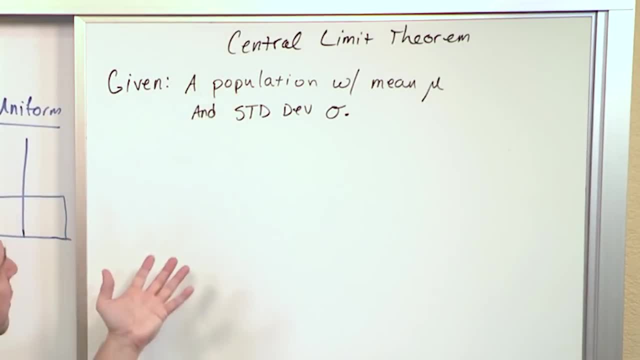 So that's given to you. We always have populations we're having under consideration. They always have a mean and a standard deviation, but we almost never know what these numbers are for real. We can't really know them. We can take surveys and estimate them, but we don't. 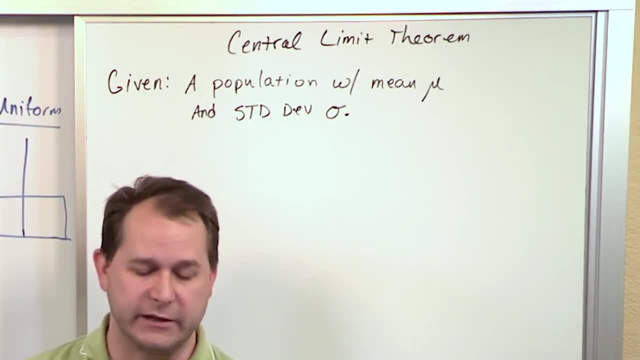 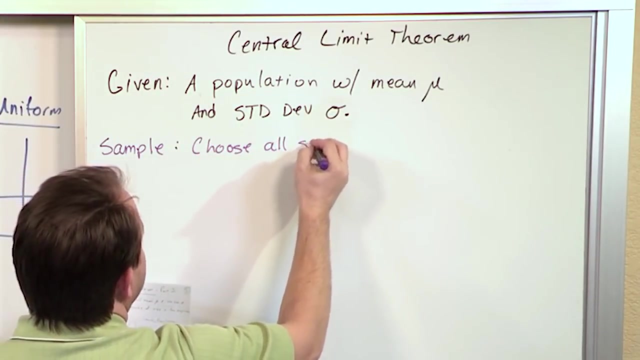 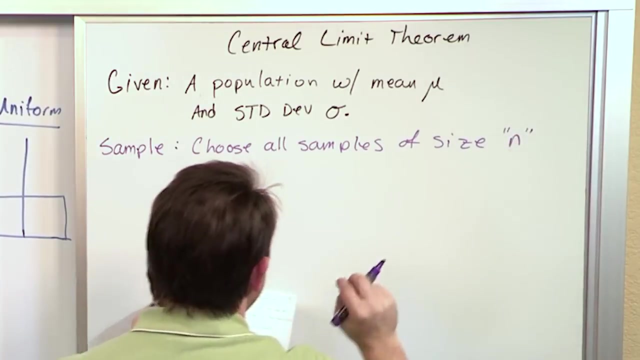 really know them, because the only way to know them is to actually talk to everybody in the country. All right, Now, underneath this, we're going to talk about sampling, So we're going to choose All, All, All samples of size n, Size n. Remember, we talked about sample size from this population. 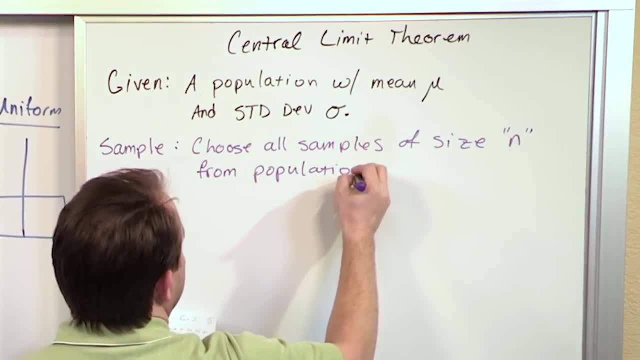 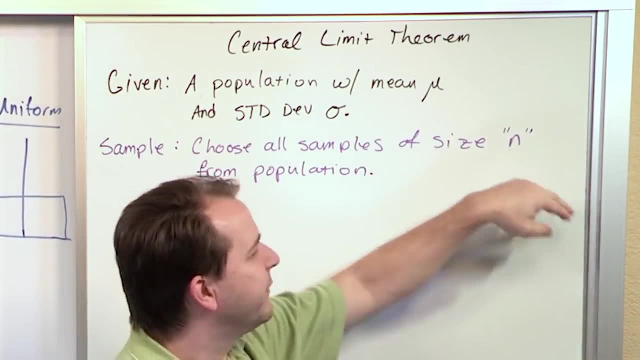 that we're talking about From this population. So if we're talking about the population being North American male boys, then we start to sample them And let's say our sample size is 10 or 15 or whatever, and we go talk to 15 people and 15 more people, 15 more people. 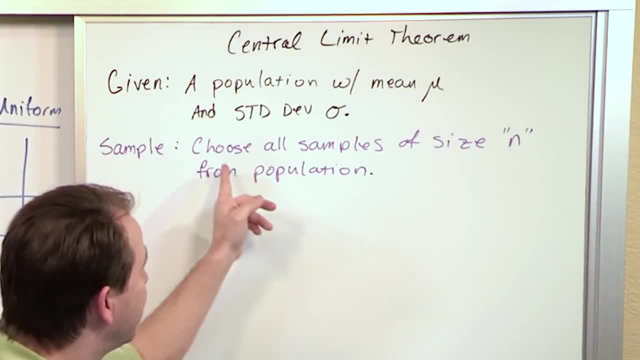 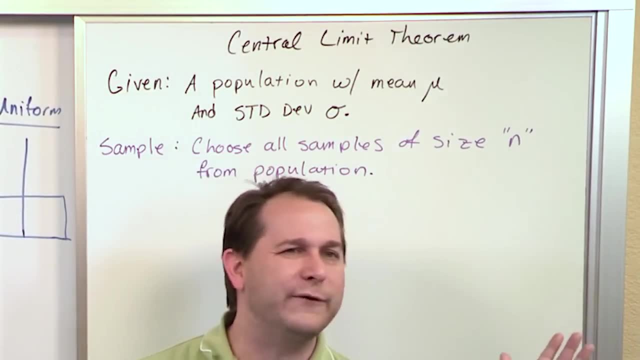 Every time we do that that's called a sample And we're doing it, Notice we're collecting all samples. So the central limit theorem: in order for it to really work theoretically, you're supposed to choose every sample from your population, every possible sample. So really, if it's everybody in North America, 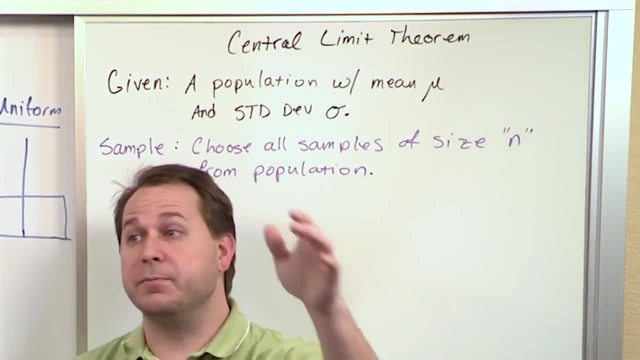 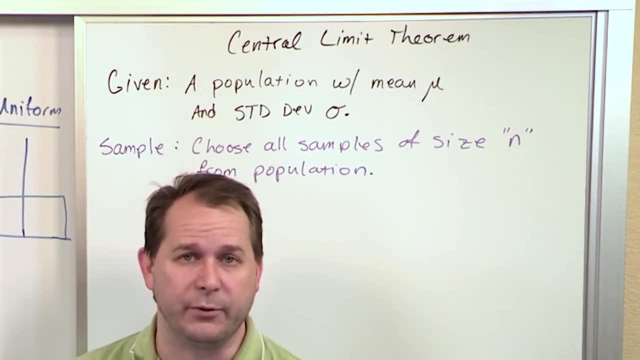 all North American males. you really are going to be taking blocks of 15 people until you've chosen everyone. Now, in practice that's not really appropriate. That's not really something you can do with that many people. But still, the central limit theorem is still very useful. 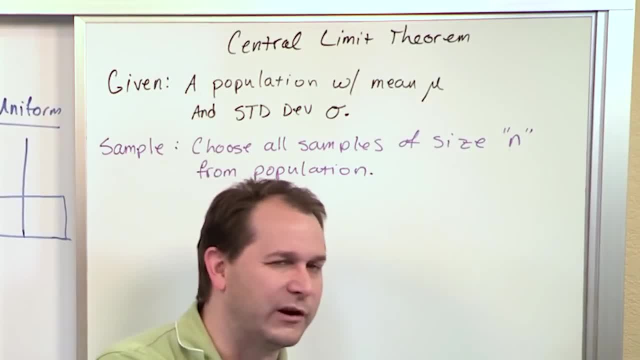 and you'll understand. Even if we're not, Even if we're not, Even if we're not actually choosing all the people to look at in the country and actually calling them all, it's still very useful. You'll see how when we do the problems. But 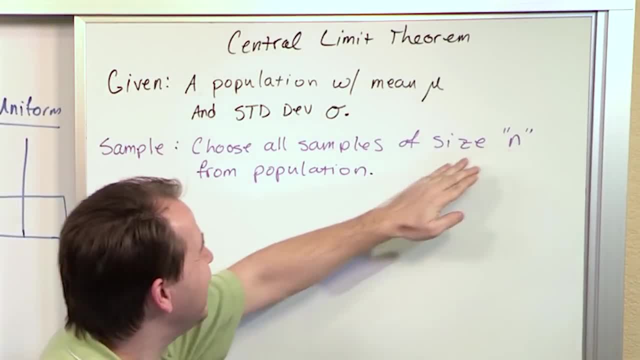 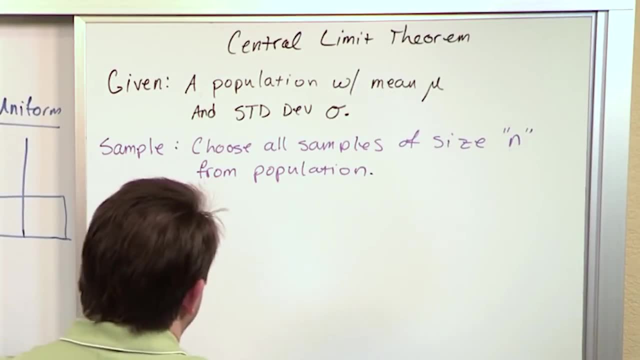 anyway, the setup is: you have a population, you start sampling of size in from the population. Now I want you to keep in mind that this population that we're actually talking about can really be any shape, And that's really the power of the central limit theorem. So normally, 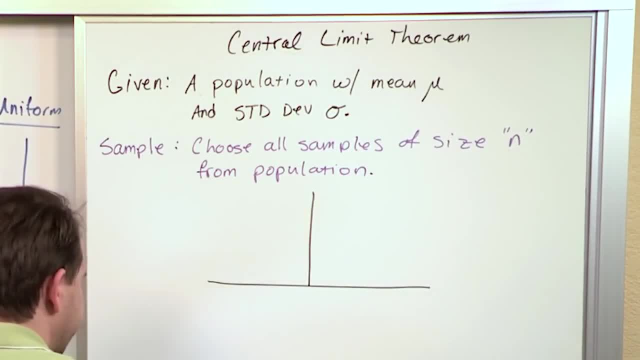 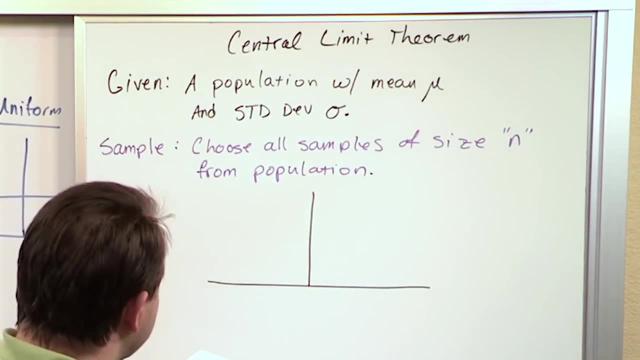 we've been talking about this bell-shaped distribution, the normal distribution. In the many, many, many, many cases, the distribution of your population is going to be the same as the distribution of your population. So the distribution of your population really does look normal. But the central limit theorem applies to any distribution, So it may not. 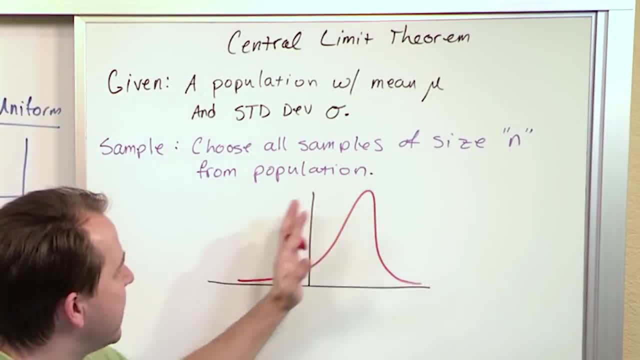 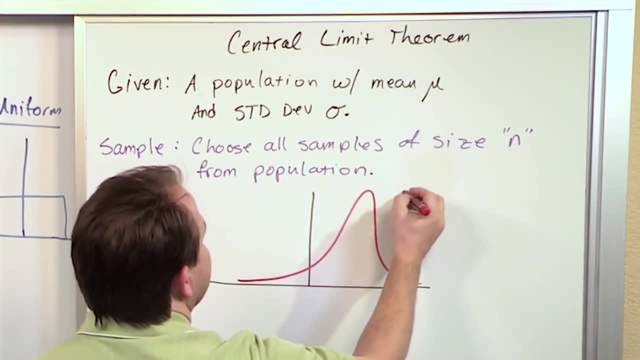 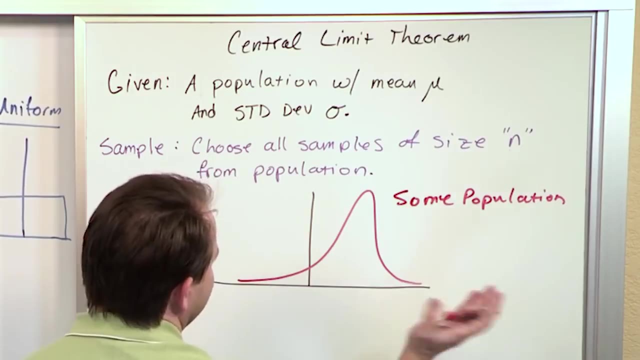 be symmetrical. It may be something like this right, So clearly the peak is not symmetric. It's pushed toward the right, It's got a longer tail off to the left and things like this. But this is some population, All right. Maybe the height of people is skewed a little bit. 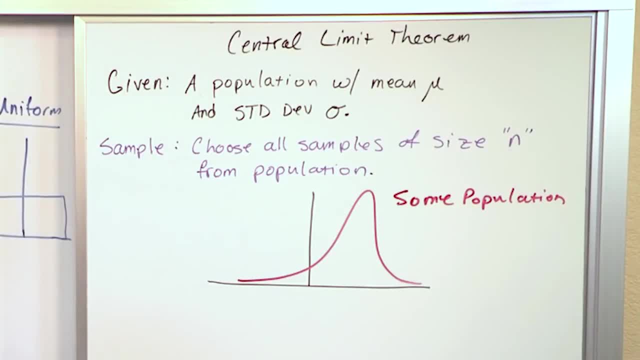 to the right compared to a nice symmetric distribution, And just to make it absolutely clear when we're talking about sampling. I'm not going to draw this picture ever again, But I'm going to do it once because I think it can really help you visualize what we're. 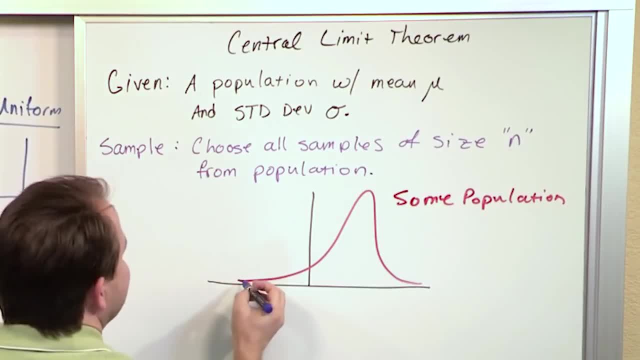 talking about. This is a population. I'm going to sample them. So that means from this population. I'm drawing an arrow from here, But I don't mean from this part of the curve, I just mean from the population. I choose a sample. I'm going to call it sample number one Sample. 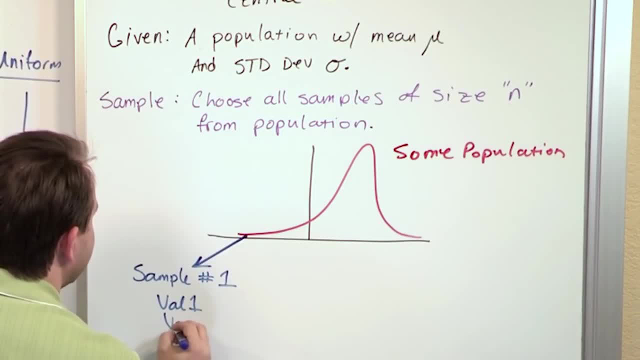 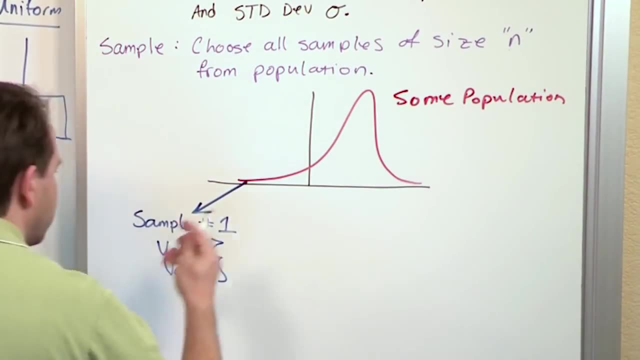 number one consists of value one and value two. Now, since I only selected two values, the sample size here n is equal to two. That's the sample size. So I get on the phone, I call two people And I say: what's your IQ? 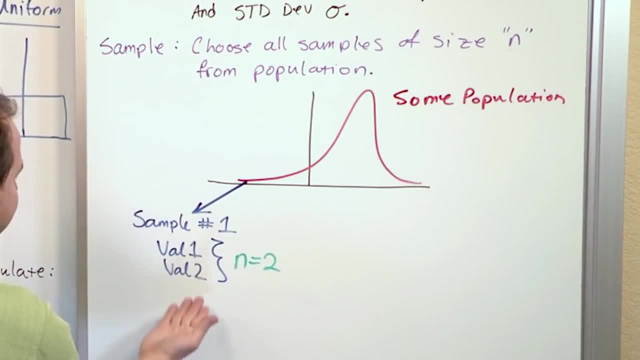 person number one: What's your IQ? person number two, And I get two answers And since I only did two people for that block there, my sample size is two And from that I can then do something. For instance, I can take this information here And I can find out. 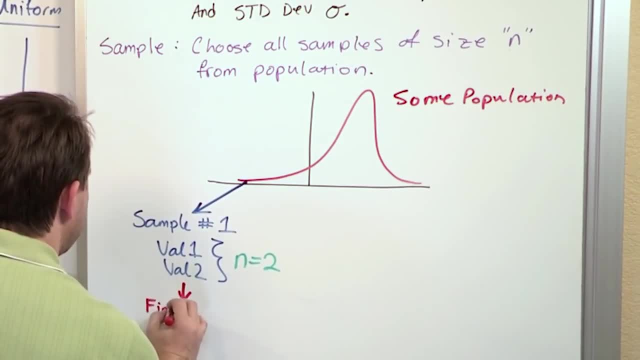 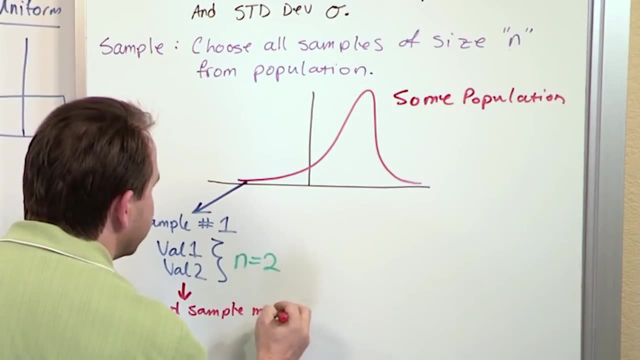 the mean, Find the sample mean. I'm using the word sample mean because I don't want you to get confused with the population mean. The population mean is everybody in the whole population Here. I'm just talking about the sample mean of the two people I called on. 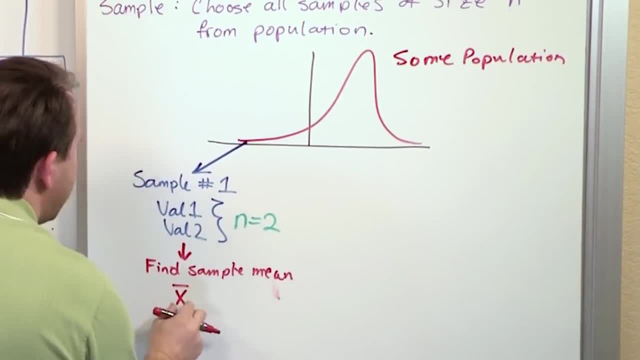 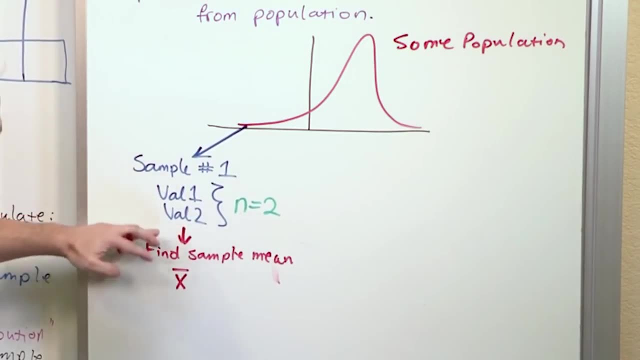 the phone. Now I denote that x bar. X means sample, Bar means average value. So this is some number. So this is an IQ. This is an IQ. I take the average value. That is sample. number one's sample mean right, OK, cool, Now I go do that process again Again. I'm 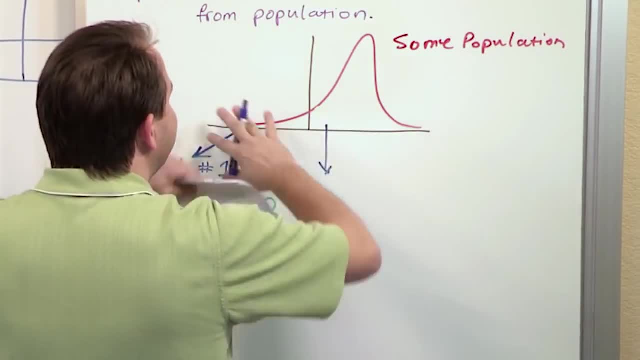 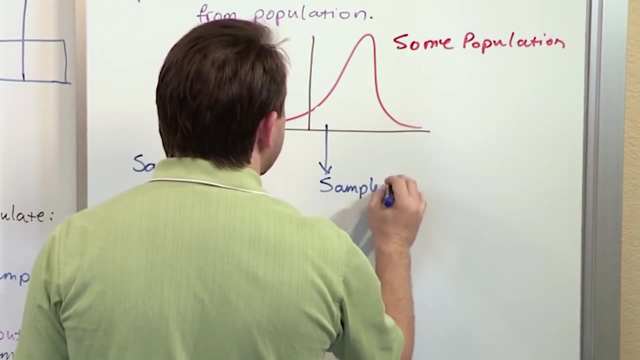 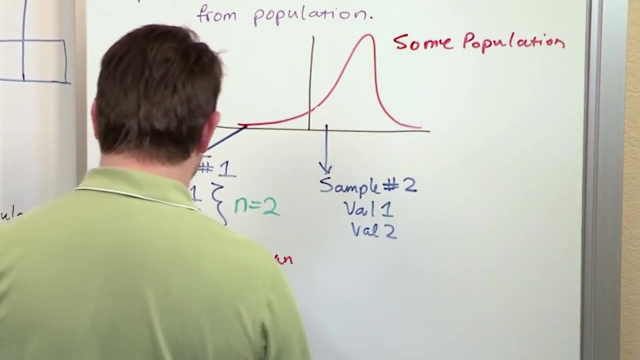 drawing an arrow from here, It doesn't mean I'm choosing from here, It just means from the population that has some distribution. I go and do the whole thing again. I say sample number two: right, And I get a value one, value two, And of course, because I only chose, 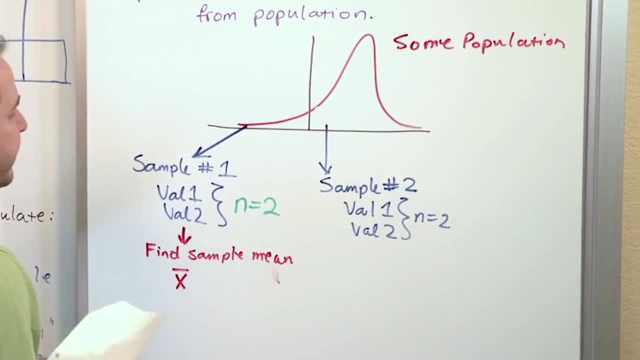 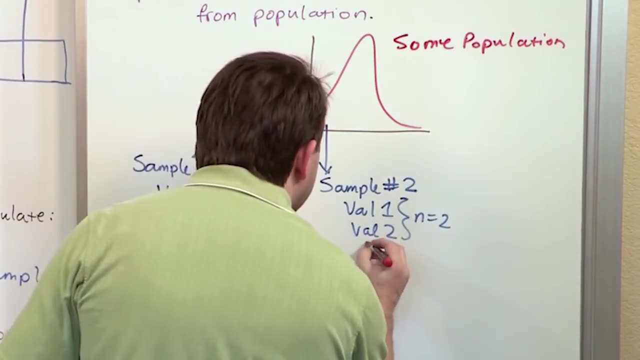 two people. n is always going to be two. Once you lock down your sample size, you're going to have a sample size. You're always choosing the same number of people for every sample there, And then I can calculate some average sample value there. some sample mean from. 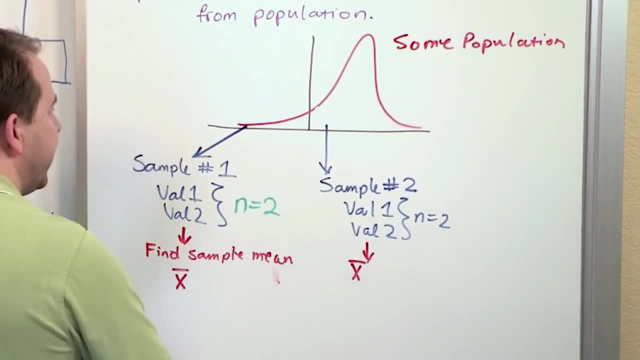 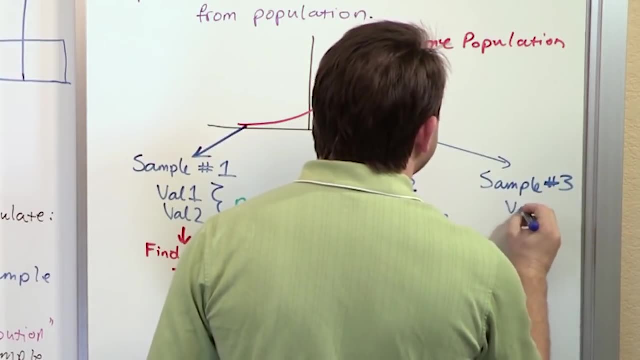 this data here, this data here that I've chosen. Now I'm not going to bore you by continuing to draw this over and over again, But just one more time. I can say sample number three: I get value one, value two. This means n is equal to two. n is always equal to two when. 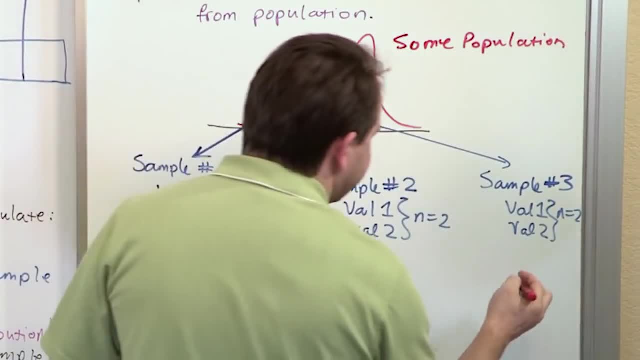 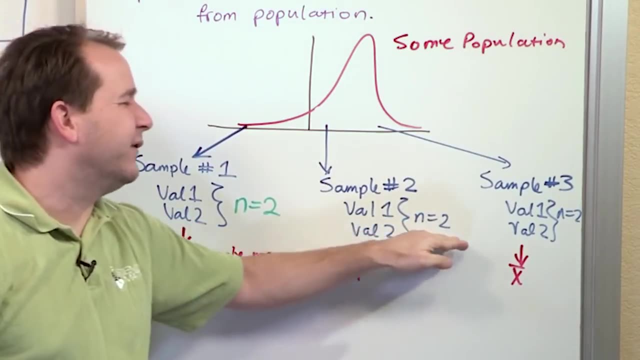 I do an experiment like this, Or I should say n never changes, And then I can calculate some average value from those data. So here I chose something simple. I said the sample size was two because I didn't want to write a bunch of junk on the board. In reality, your sample size is always larger. 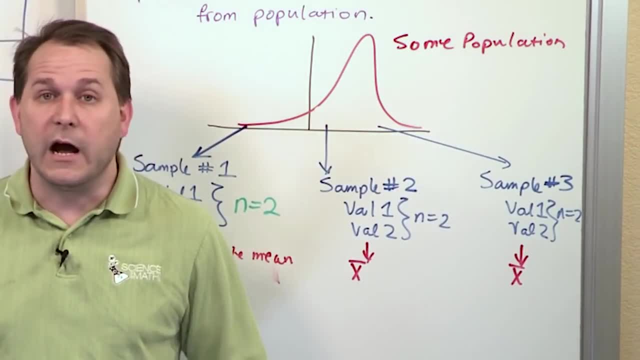 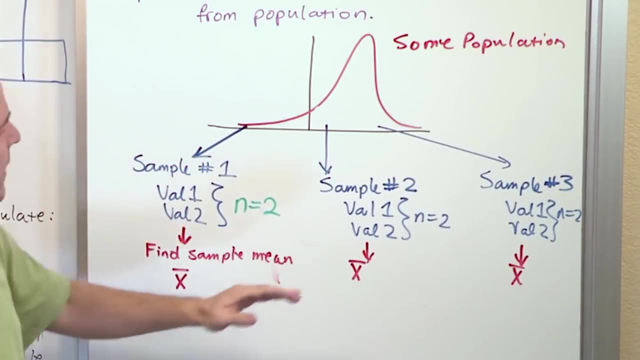 than two. Your sample size might be 20 or 30 at a time, for instance, in which case I would have 30 values And I would take an average value and get x-bar for sample number one. I would get 30 more values and get x-bar for sample number two. I would get 30 values. 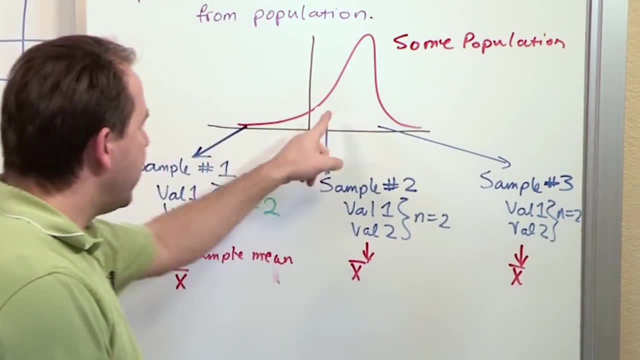 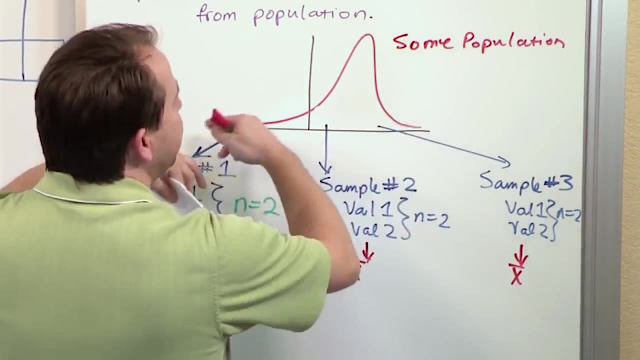 for x-bar, I would get 30 more values for sample number three. I'm drawing the arrows out of this curve, not trying to tell you where this data is coming from, but simply saying that each of these samples come from a population which is not necessarily normal, not necessarily. 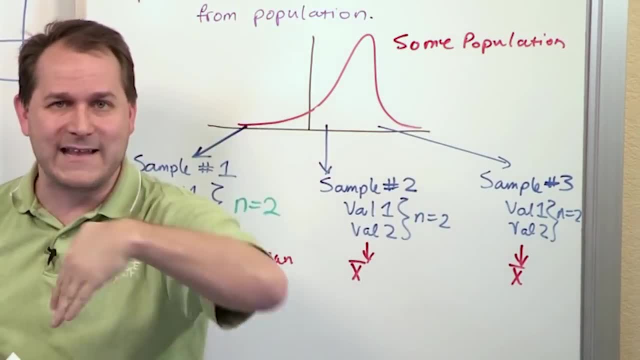 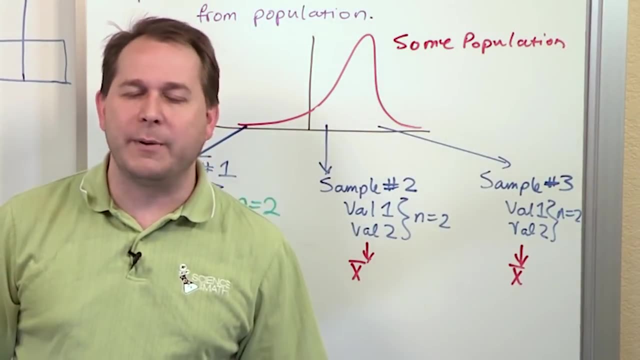 symmetric. In fact, this could be a uniform distribution with just a flat line. It doesn't matter what you're sampling from for the central limit theorem. That's actually why it's so useful, Because we don't know in real life what the population really is. We have guesses. 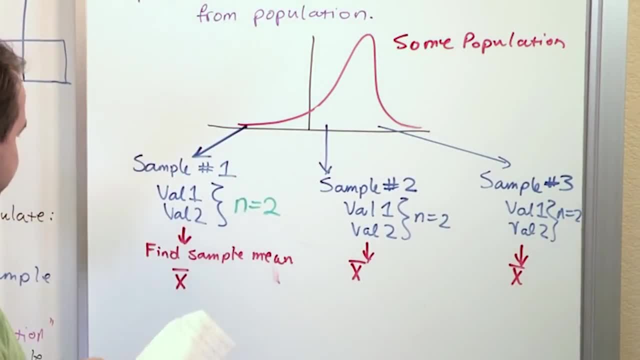 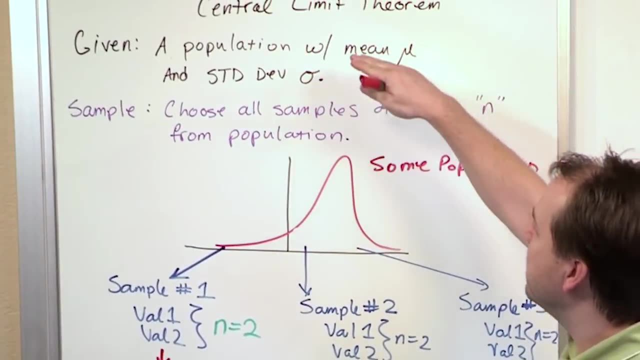 and stuff, but we don't really know. Central limit theorem doesn't care, So let me scoot this over here And now let's finally talk about what central limit theorem is. This is the setup. The central limit theorem says I'm given a population, It has a population, mean and a population. 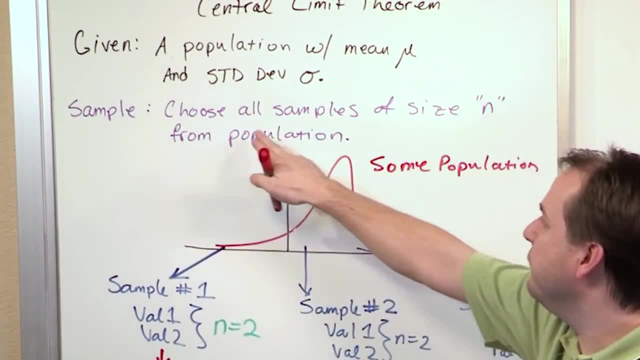 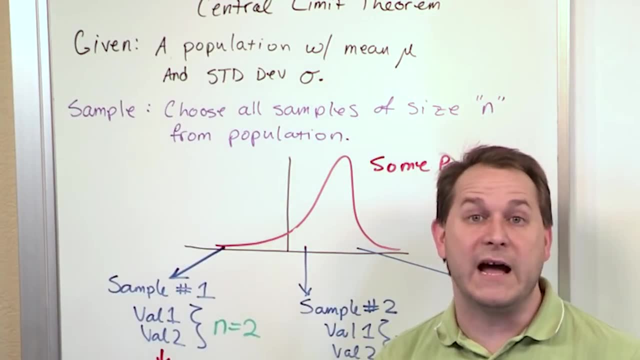 standard deviation. I sample from this population by choosing all samples of size n from the population. So I do sample number one, sample number two, sample number three, sample number four, sample number five, each time collecting n number of data points, calculating something. 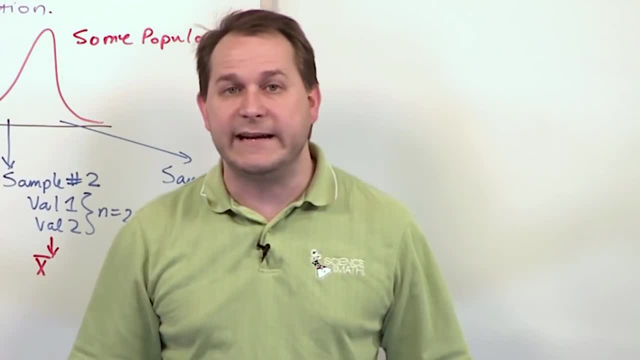 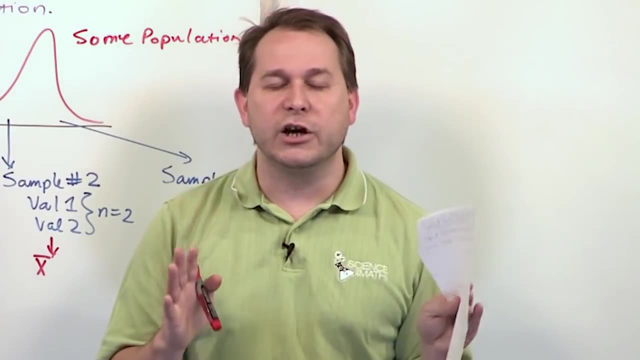 from it, And I keep doing this, doing this, doing this until I've basically sampled the entire population. Whatever I've defined that population to be, I've got a bunch of data at that point. Now what follows is the conclusions you can draw from that data. Keep in mind the population. 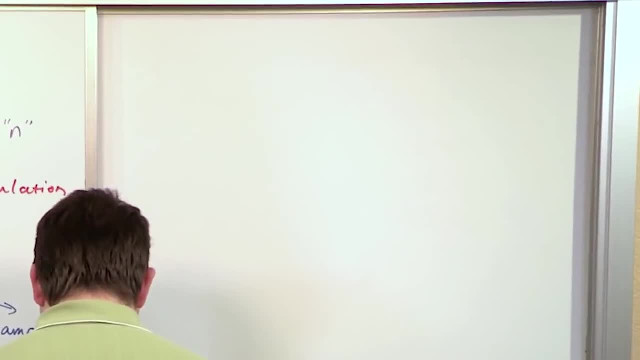 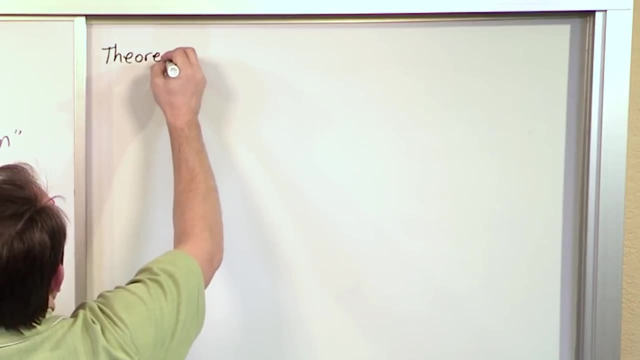 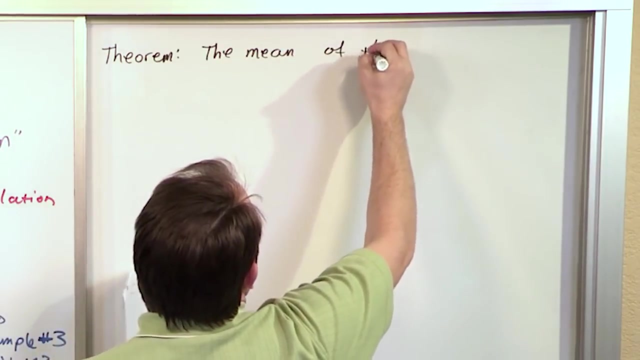 I'm sampling from doesn't matter what the shape of it is, All right, So we're going to draw what this is. This is actually what the central limit theorem is, So I'm going to put theorem. The mean of the sample means n, So I'm going to put the mean of the sample. 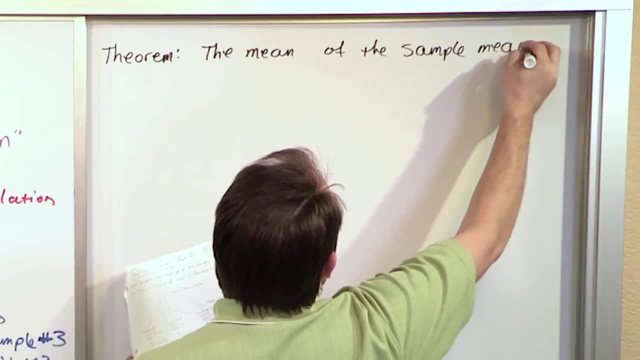 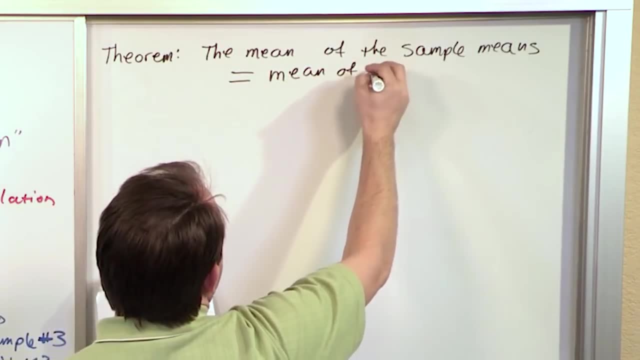 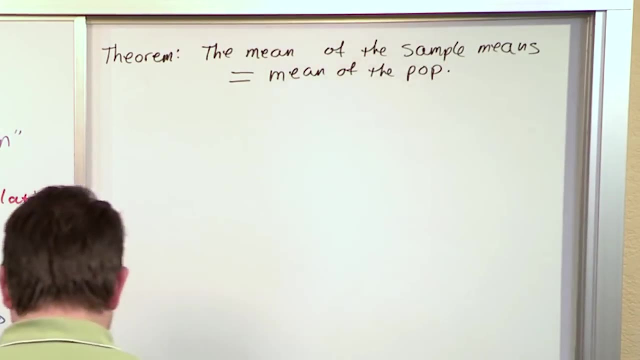 mean- I don't know if this looks weird, but I'll explain in a minute- Is equal to the mean of the population. The mean of the sample means is equal to the mean of the population. That's a lot of means in one sentence. I don't like that, but I have to do it because that's. 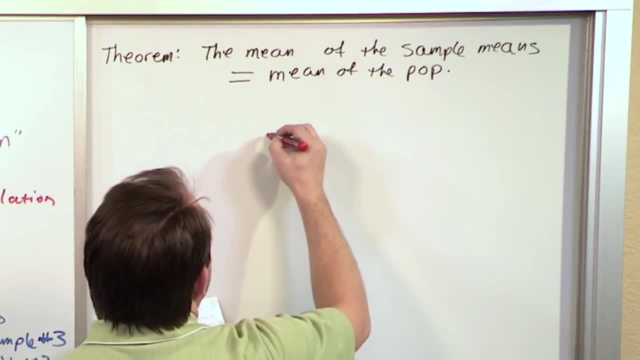 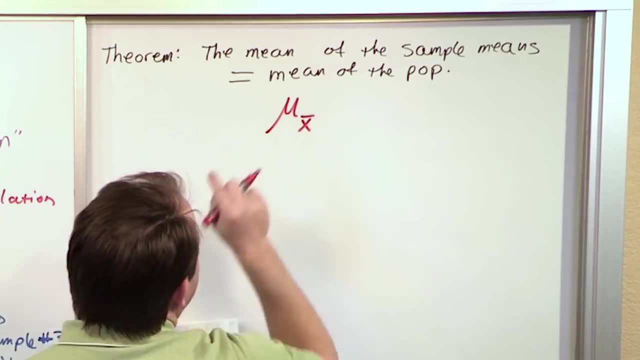 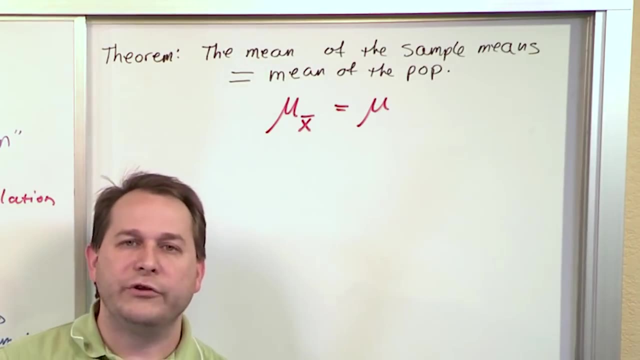 the way it's defined. The way you write this is you say the mean of the sample means. Remember the x bar is the sample means. that I've done. If you take the average value of all the sample means, it's equal to the mean of the entire population. It doesn't matter what your sample. 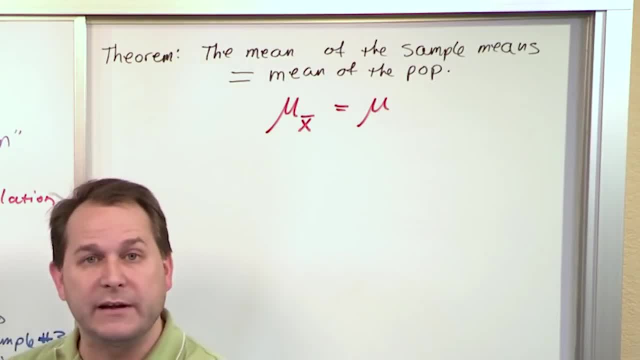 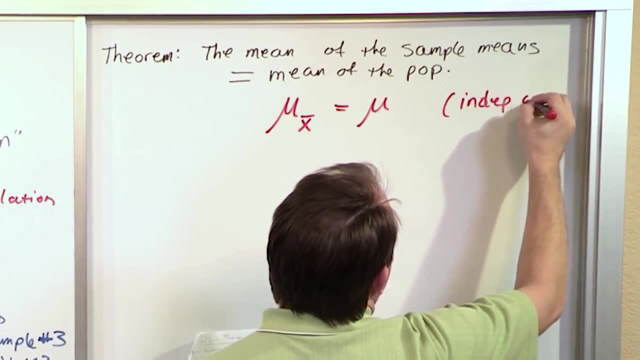 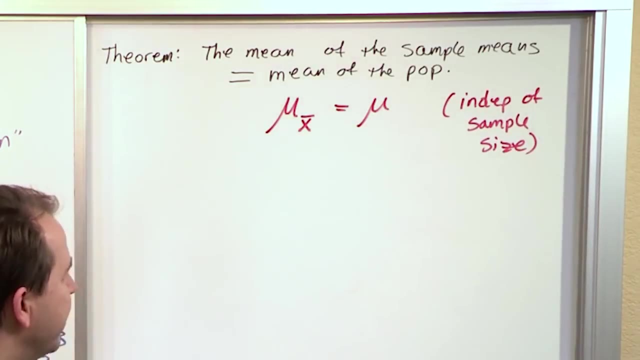 size is. It doesn't matter what type of population it comes from. So I'm going to put in parentheses: independent of sample size. This is actually quite remarkable, But you know it's not that crazy when you think about it, What this is basically saying. let's go back to our drawing. 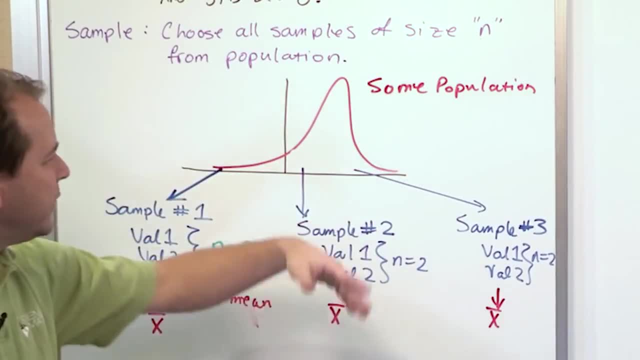 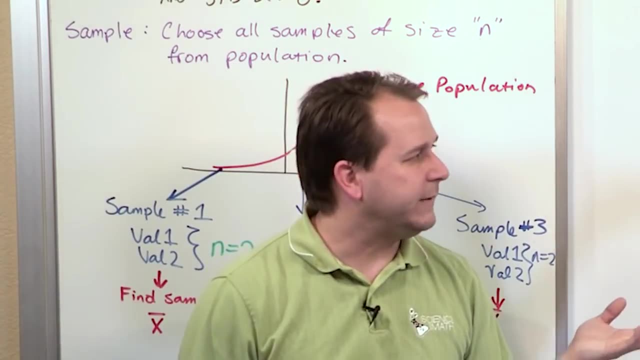 What it's saying is: here's a population. I don't know what the shape of it is. I take sample, sample sample. I calculate the average IQ of every sample. Let's say we're studying IQs, All right. So here I have a data point from this sample, which is the average IQ. 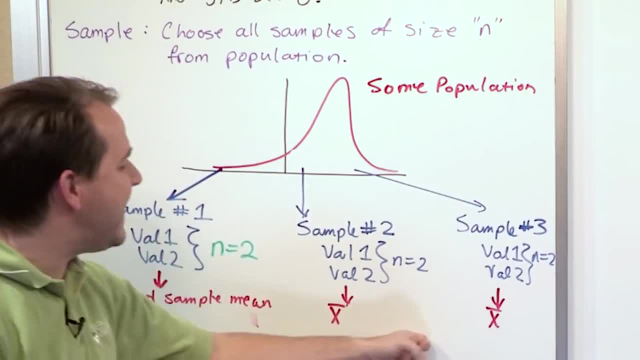 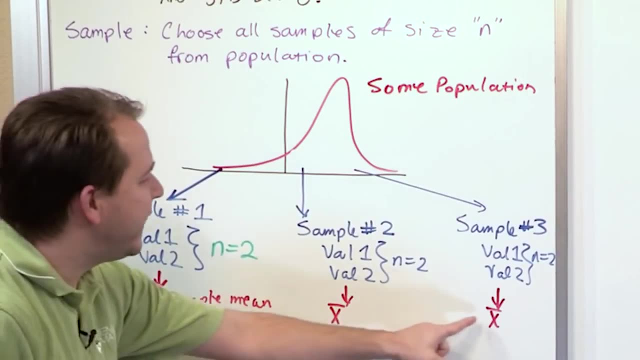 The average IQ here, the average IQ here for every sample, If I take the average of all of the sample, means, in other words, the average value of this plus the average value of this if I add them all together. in this case, if I only have three samples, if I add them. 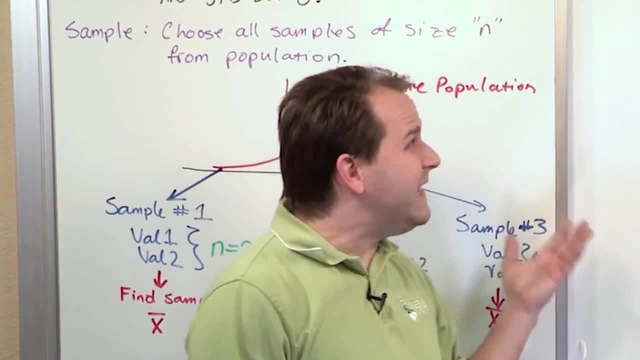 up and divide by three, I'd be finding the average value of this plus the average value of this. Let's say I take the average value of the sample means- right, Because each one of these is called a sample mean. If I take the average value of all of those, I get the mean of the. 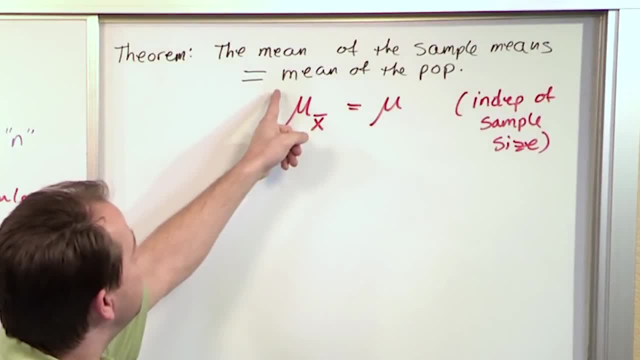 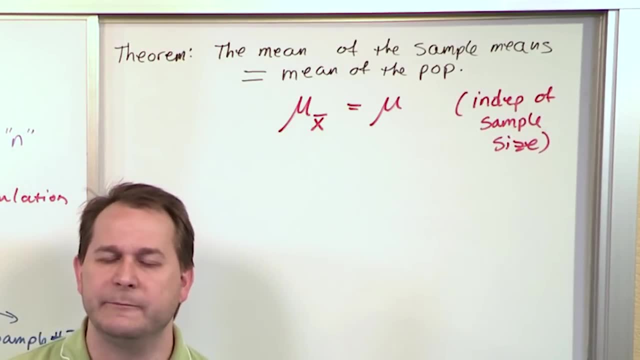 sample means. The mean of the sample means is equal to the mean of the population, Right? So what it's saying is: okay if I don't know anything about the population, if I go and sample the population, right, if I go and sample the population and I collect all of. 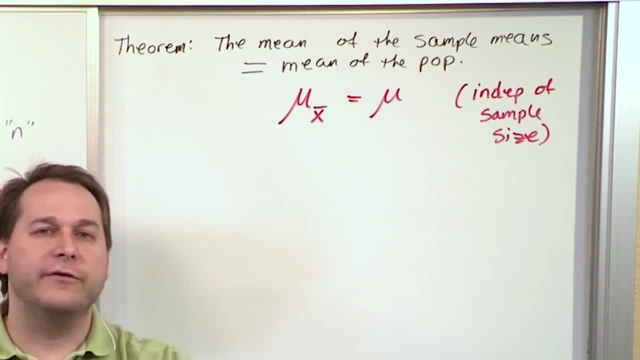 the sample means right, and then I average those values. what I get from the sample means what I use. what I get is going to be exactly equal to the mean of the population, And it doesn't matter the shape of the population and it doesn't matter how many samples are. 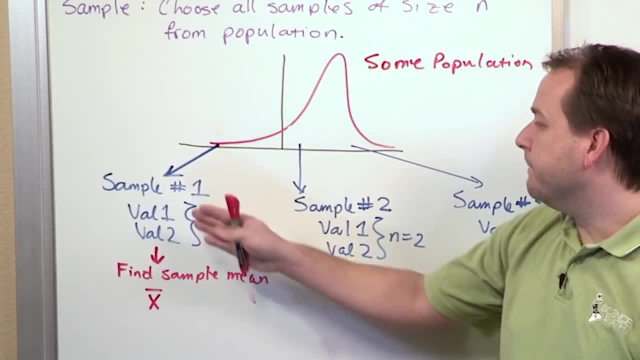 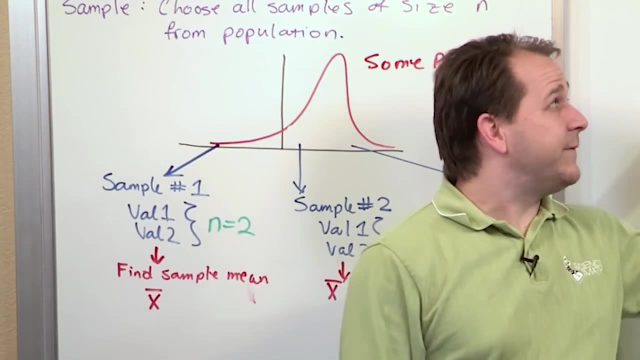 in, or what n is, how many samples are in, or the sample size is what I'm trying to say. The size of the sample doesn't really matter whether I'm collecting two values or ten values. Now, this is definitely pretty powerful, but there's a couple of gotchas that make it a 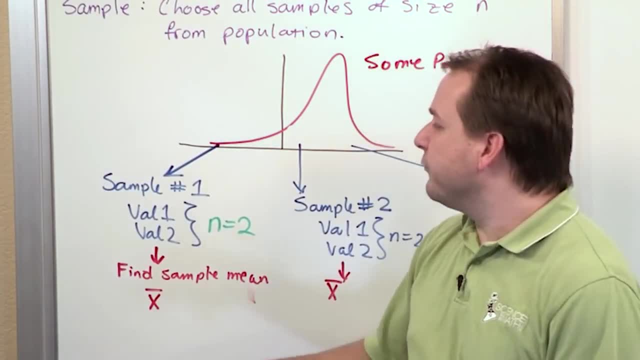 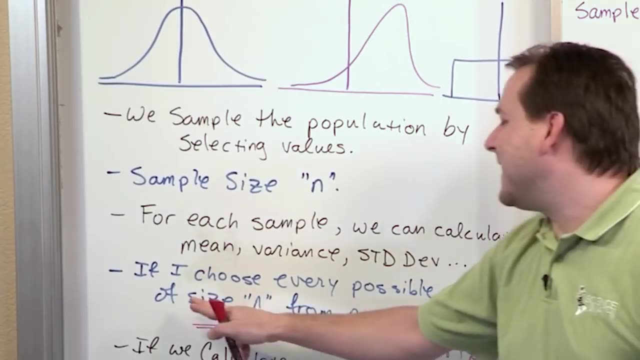 little bit like well, who cares too much? Number one is the central limit theorem is basically assuming that I choose every possible sample of size n from the population. That means that I literally have to collect all the data, So it isn't terribly surprising. 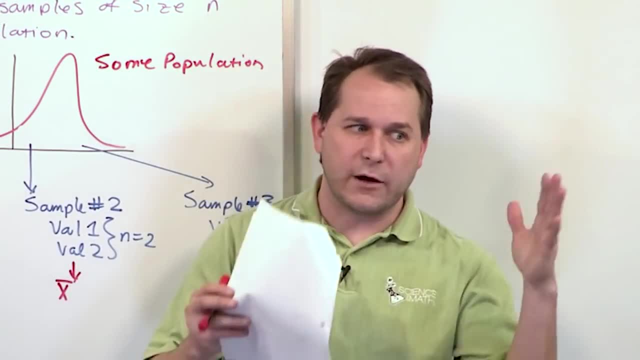 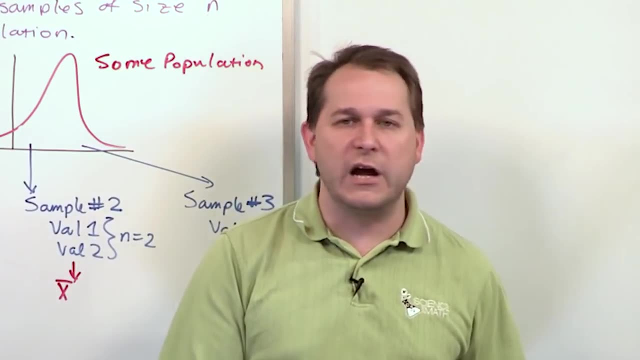 that if you collect all of the data from the population, and if you collect all the sample means and then average them, the answer that you get should be the same as the population mean, because, in effect, what you've done is you've averaged small groupings of data points. 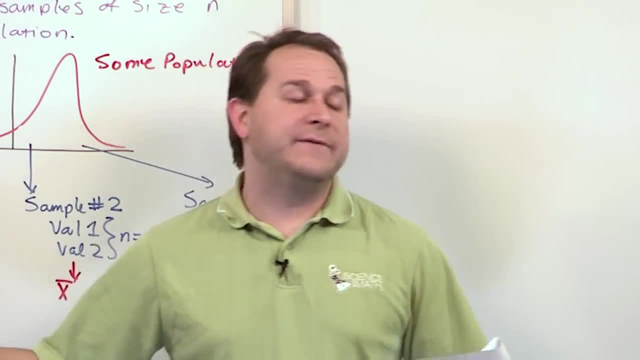 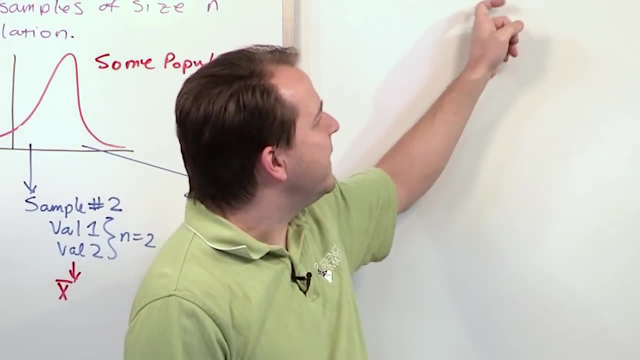 got those numbers and then you've averaged them all again. But since you have to cover everything in the population, you've basically collected all data points and averaged them, And that's telling you that what you get here, if you average the sample means, is you're. 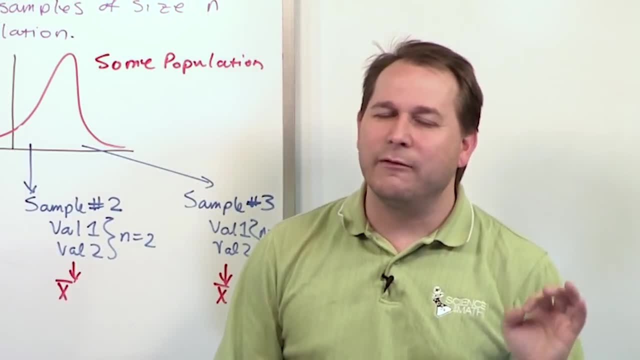 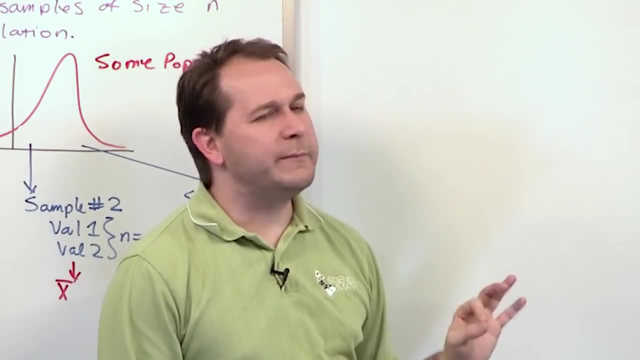 getting the same thing as the population mean. That part's not terribly surprising. The next part that we're going to study is a little bit more surprising. This is not terribly surprising. However, there's a couple things. The central limit theorem is defined and derived. 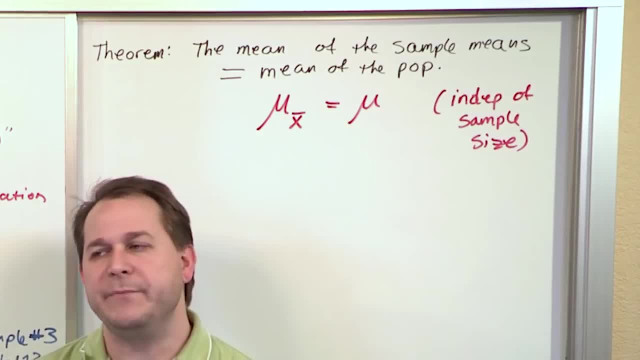 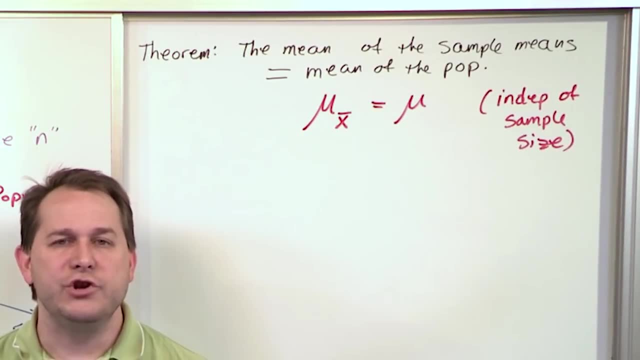 in terms of sampling everything from the population, But in real life you can't really do that. So what really happens is, if you choose a sufficient number of samples right and you do that, then you can get pretty close. You get a pretty doggone good estimate of the. 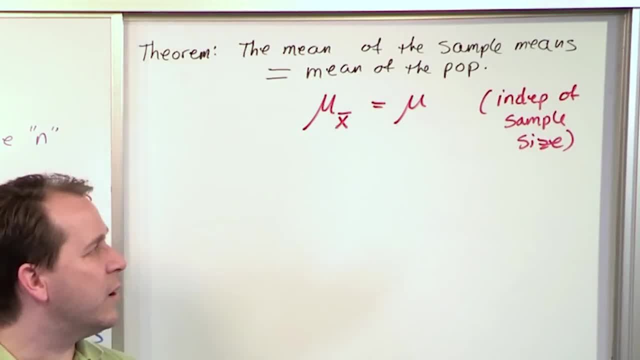 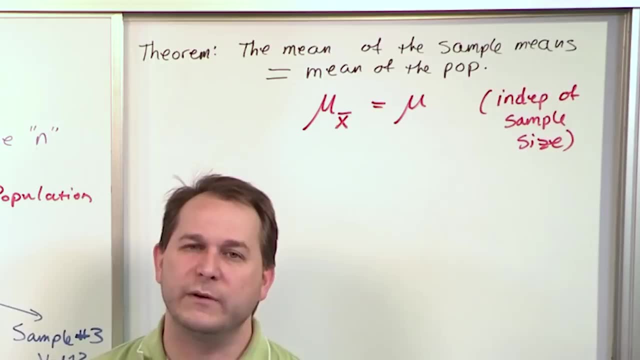 population mean by just taking a large number of samples. So even though this doesn't seem too remarkable in theory, because you have to choose everybody, it still has utility. It still has value, because what it's basically telling you is: it doesn't matter the shape. 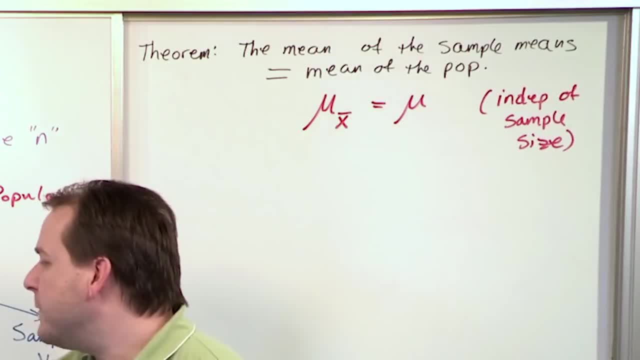 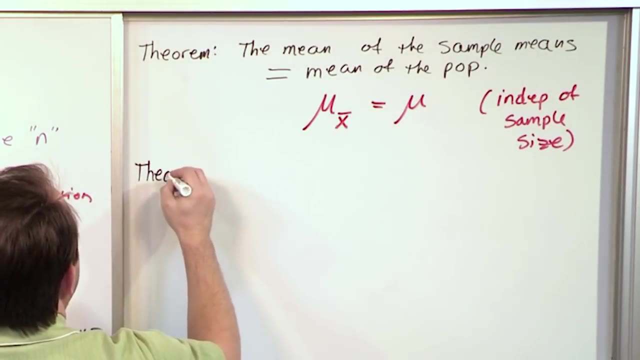 of this distribution. If you sample enough times and you average them and you take the average of the sample means you're learning something about the population that you didn't know before. right, That's important. All right, The next thing we're going to talk about, I'll write the word theorem. This is all. 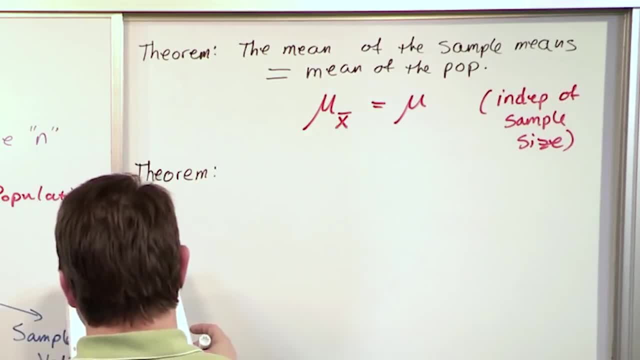 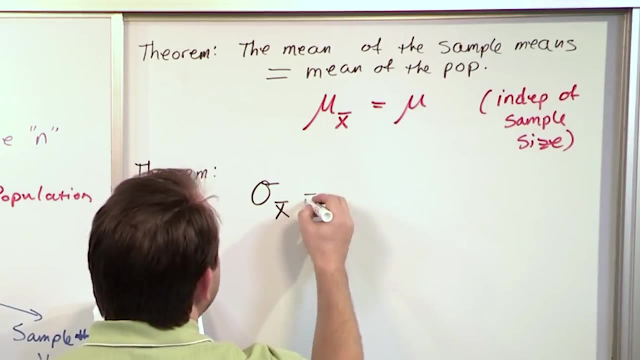 part of the central limit theorem. It's got like four or five parts to it. I'm just going to write this down Instead of writing down a bunch of words. I'm just going to write down the equation. The standard deviation of the sample means is equal to the population. 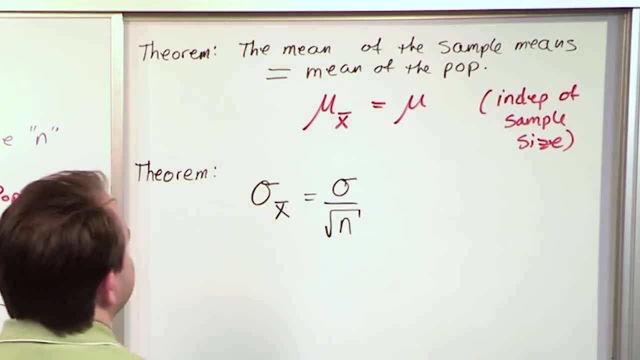 mean divided by the square root of n right. So what it's basically saying is that the standard deviation of the population means is equal to the population mean divided by the square root of n right. So what it's basically saying is that if I calculate the 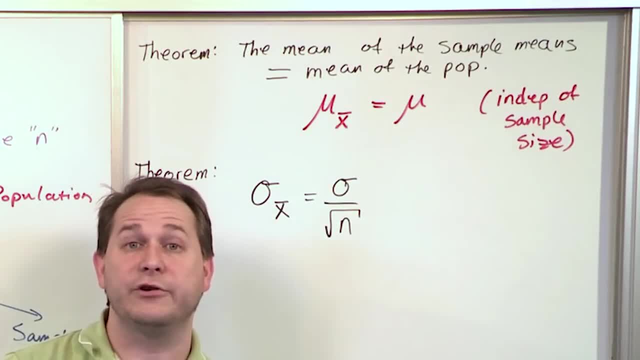 sample means, all these X bars, sample number one, sample number two, if I calculate the sample means and I go find the standard deviation of that data, which you can do easily. we've learned how to calculate standard deviation of numbers in the past. sets of numbers then. 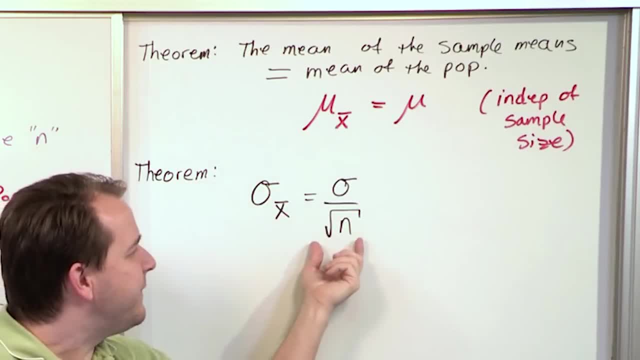 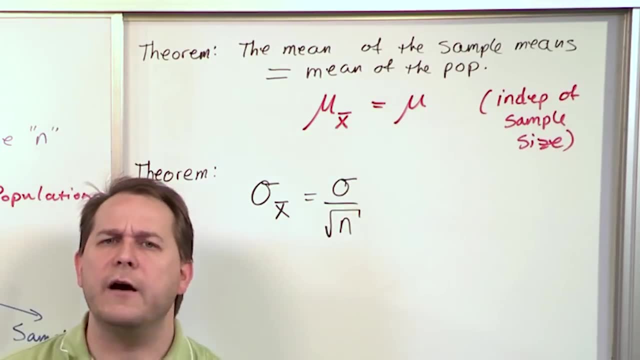 I have what's on the left-hand side of the equation that comes from my sampling. If I know what the sample size is- let's say the sample size is 10, then I know what this is. What it's telling me is I can calculate the standard deviation of my population just by 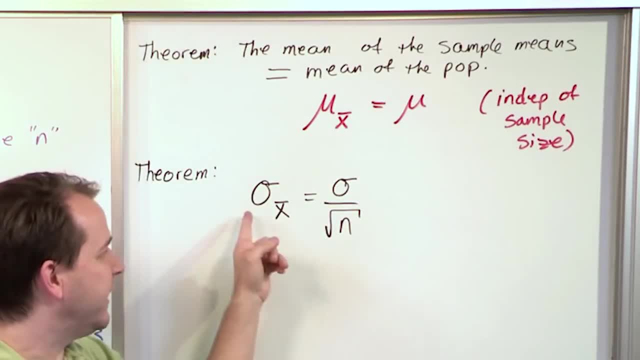 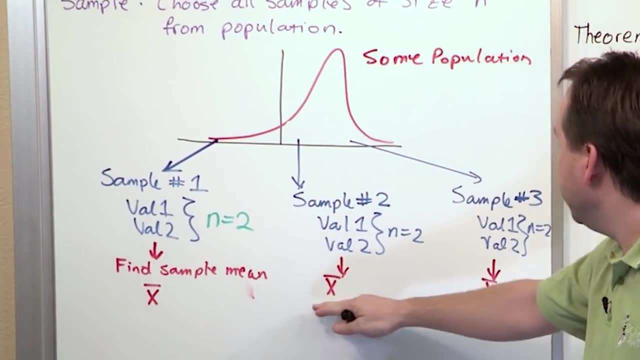 sampling data, okay, and calculating this stuff here. So what really would happen is you get on the phone, you collect all your information Here. I've got a sample mean, a sample mean, a sample mean, and so on. I've got my raw data that I've collected from. 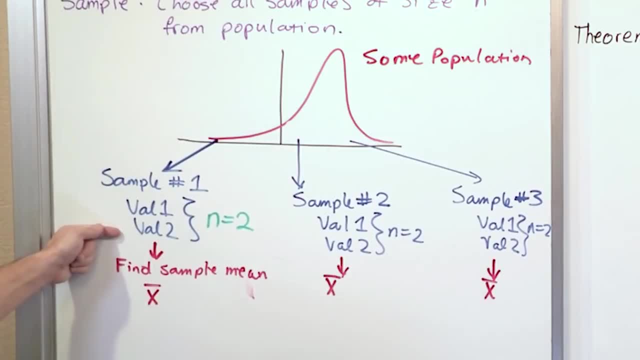 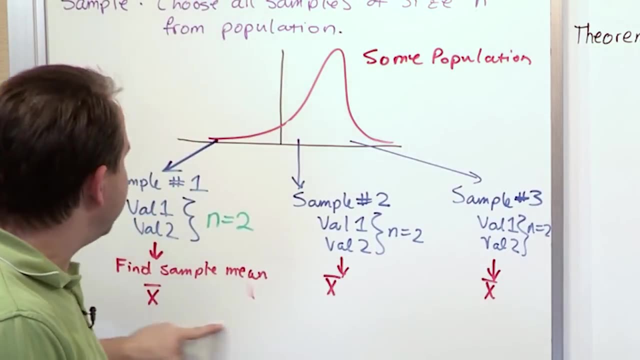 each of my samples. Now, if I calculate a standard deviation, or I should say, if I find the sample mean here, the sample mean here and the sample mean here, and I put these numbers for all of my samples into the equation to find the standard deviation, I'm going. 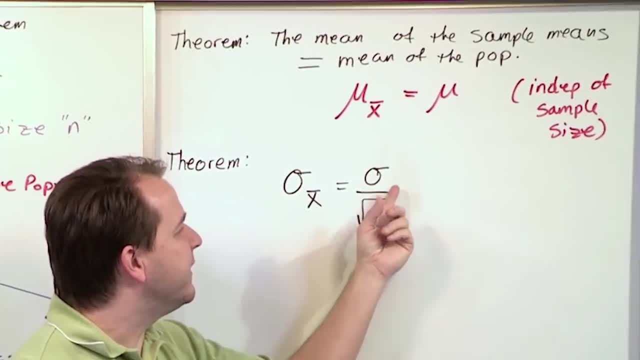 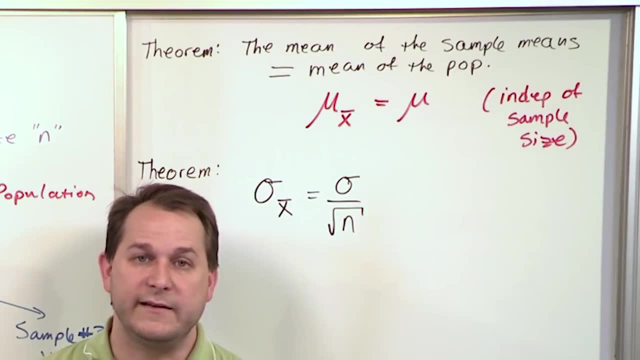 to get what's on the left-hand side, And once I know that and I know this, I can calculate the standard deviation of the population. Now, again, same kind of caveat I want to just point out to you is that it's we're set up here so that, in order for this stuff, 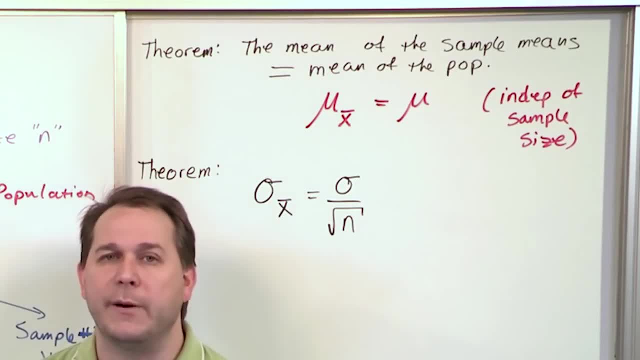 to be true, you really need to be sampling the entire population until you've exhausted all possible samples. So you select 20 people at a time until your whole population is sampled. all right, So it's not that remarkable, okay, that that you can do something like. 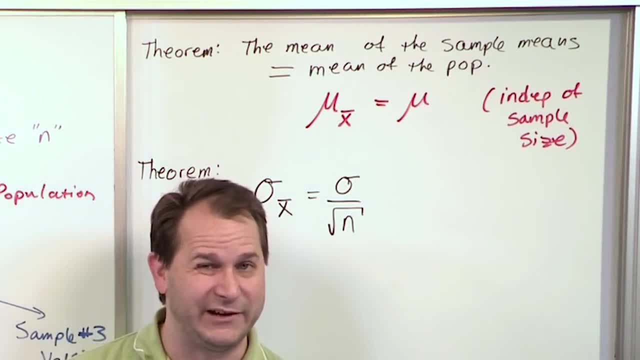 this because, to be honest with you, if I selected all possible samples of my population, then I can just calculate this directly. I can calculate the standard deviation of that data directly if I want, But still, in reality, even if you don't sample everybody, all right. 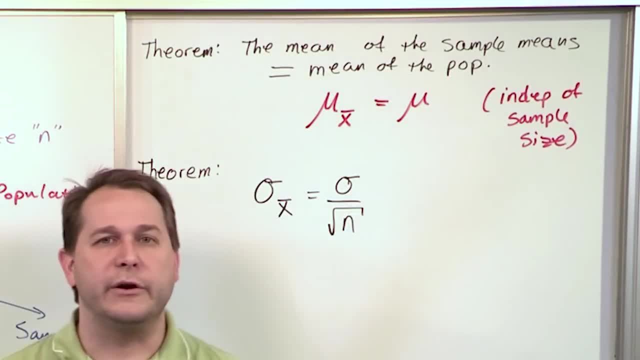 you can still get closer and closer and closer to the true value here if you just do a large number of samples. So in practice you'll just do a very large number of samples and do the best that you can to get close, to calculate as close as possible to calculate the standard. 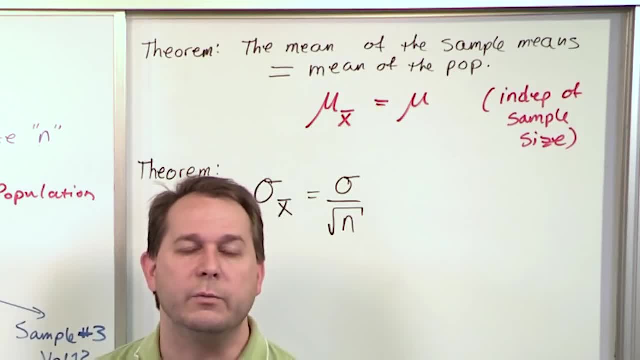 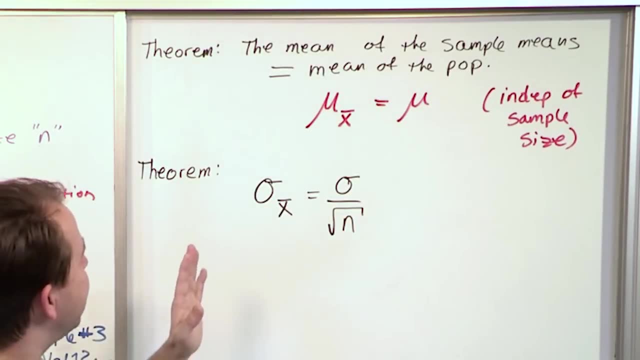 deviation of this value, And we'll talk a lot about how to do that later on when we talk about confidence intervals, but I'm kind of laying the groundwork here as we go. The most important thing for you to realize is that when you collect your sample means in this: 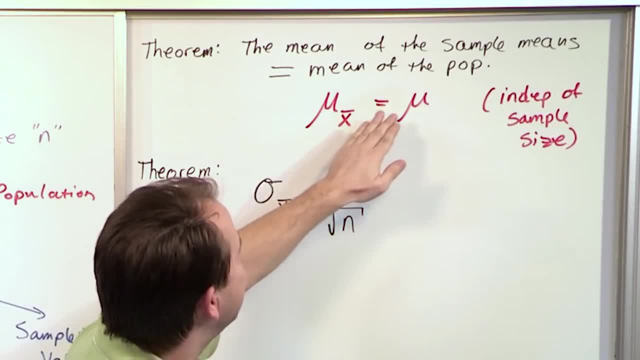 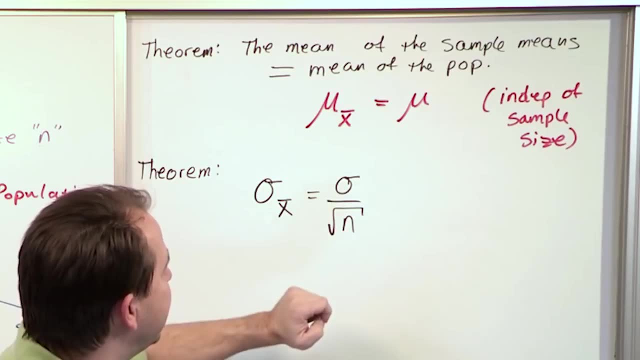 case, if you take the mean of the sample means it's going to always equal to the population mean And if you take the standard deviation of the sample means it can be related to the standard deviation of the population. Of course there's a factor down there in the 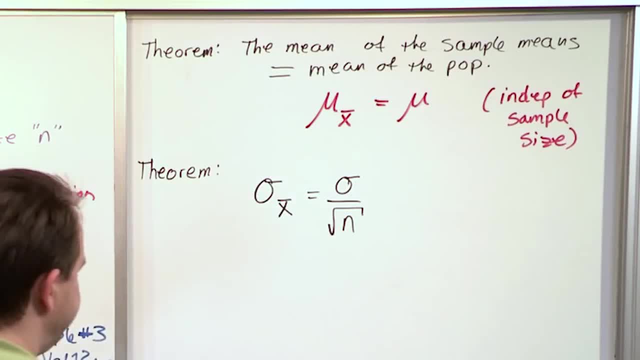 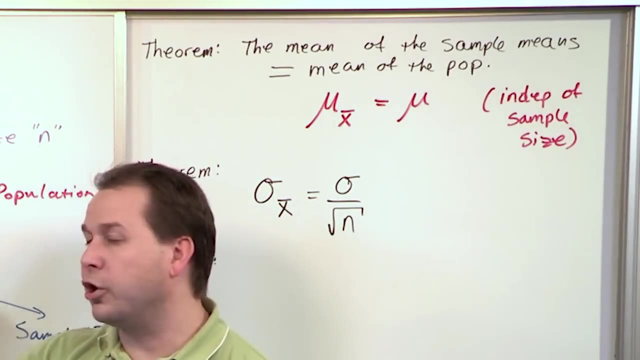 bottom, but basically it's related. Okay, Now the next thing I'm going to write down: if now, so far, this stuff is really applied, It doesn't matter what type of population curve. my original guy is Here, it's skewed. 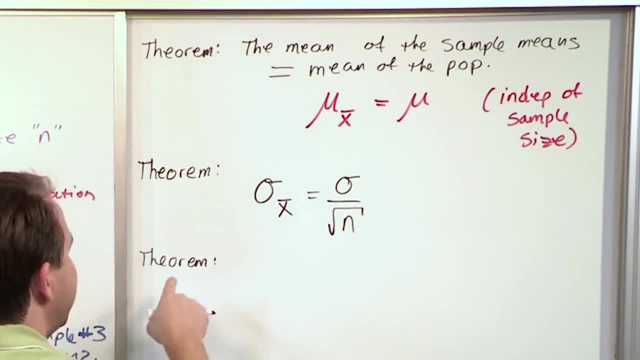 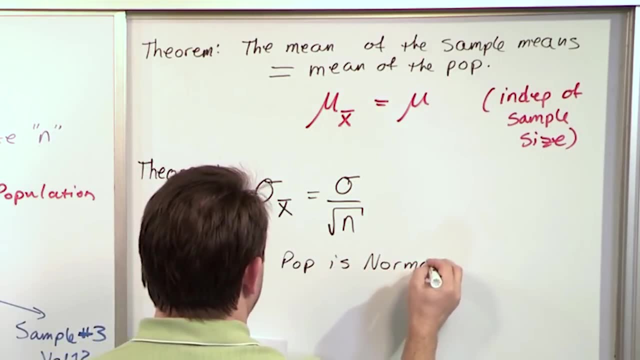 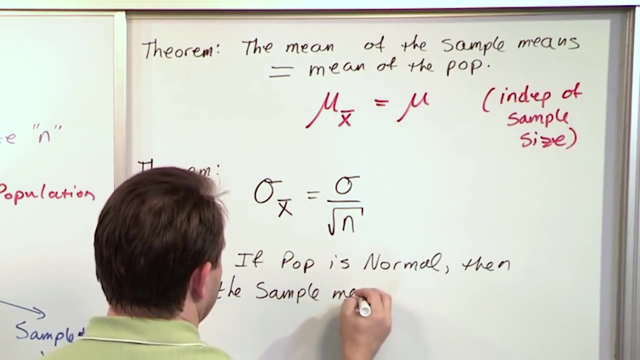 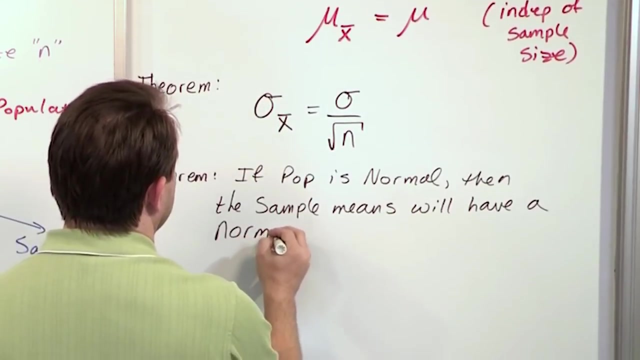 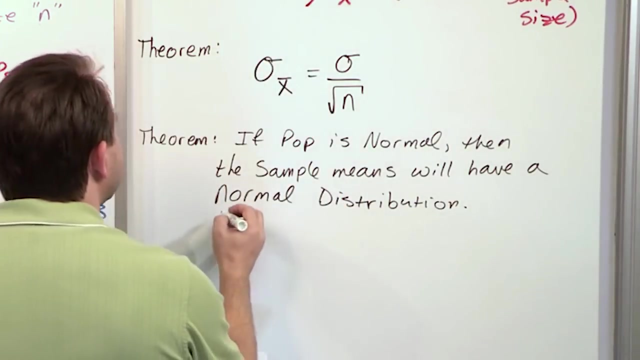 It doesn't matter, It could be uniform, It could be something else, All right. But here in this part I'm going to say: if the population is normal, Then the sample means will have a normal distribution And this is independent of sample size. 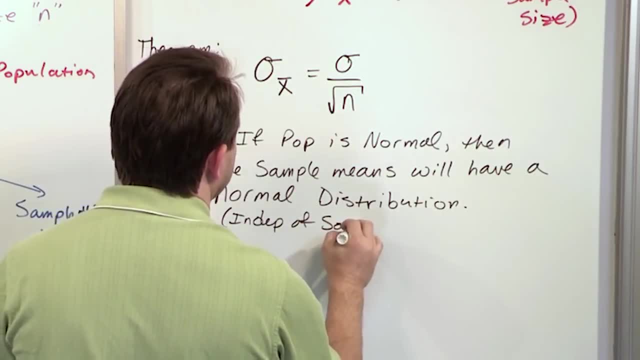 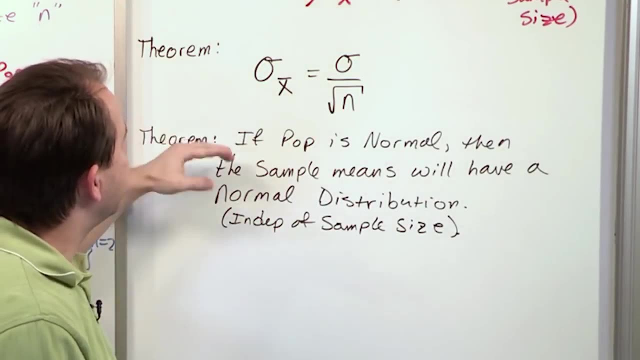 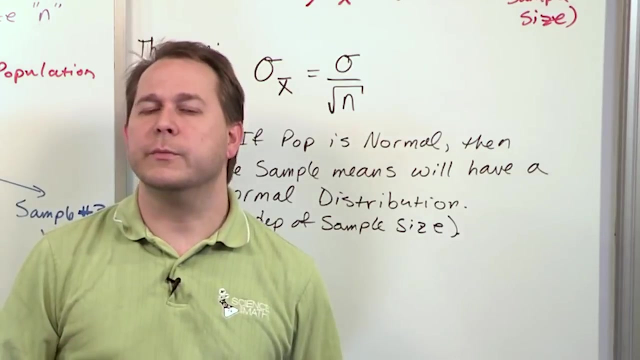 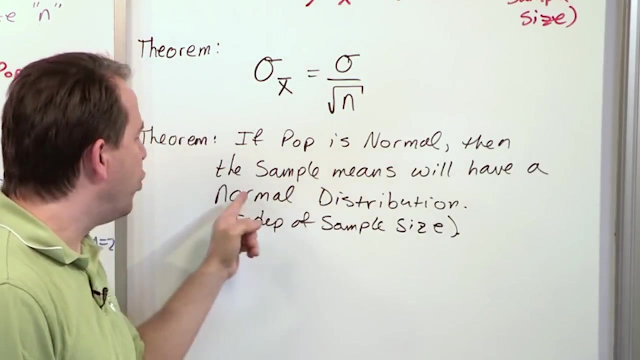 All right, The central limit theorem has several parts. The first two parts we've talked about. The third part's now narrowing the scope a little bit. It's saying now, if we assume that the population really is a normal population, then the sample means that I have calculated there will form a. 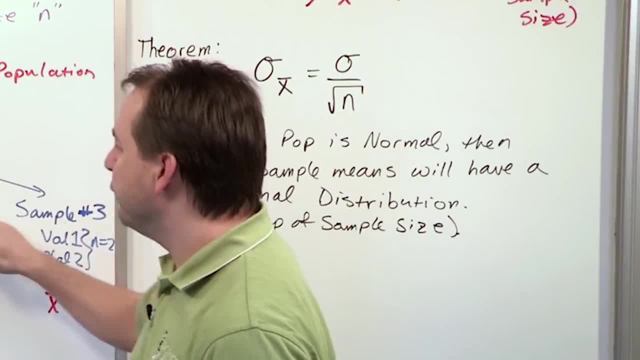 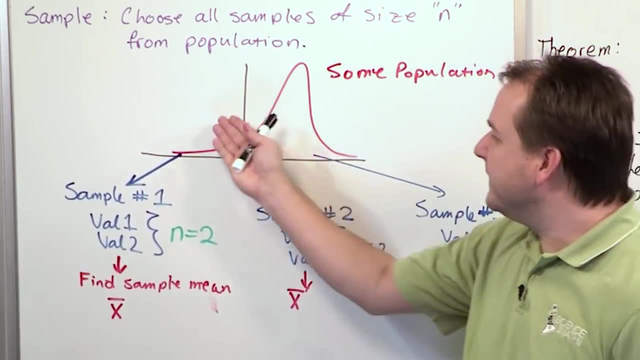 normal distribution themselves. This is why I actually drew this picture, because I want you to have a mental image. If you start throwing these terms around without an image, you don't really know what they're talking about Here. if you take sample number one, calculate a sample. 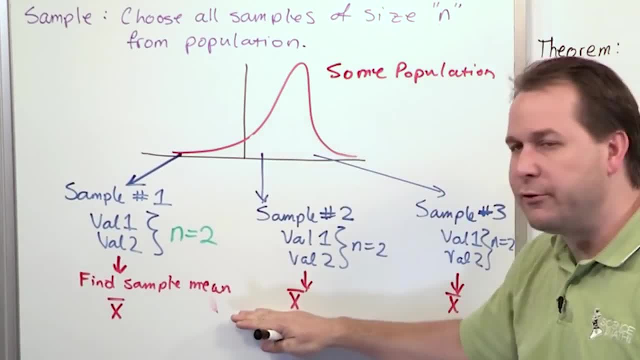 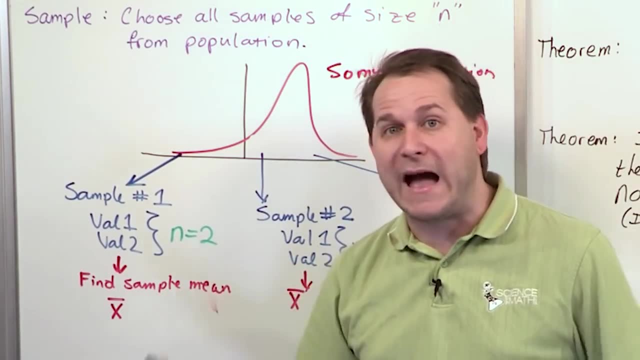 mean right: Sample number two. calculate a sample mean Sample number three. calculate a sample mean Sample number four. sample number five. sample number six: sample number 1,000, sample number 2,000.. You calculate a sample mean for every one of those things. If my parent population. 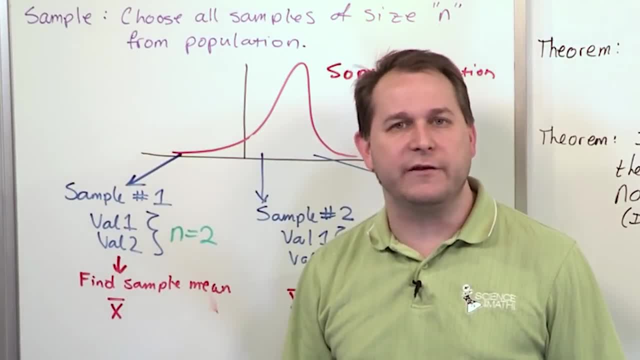 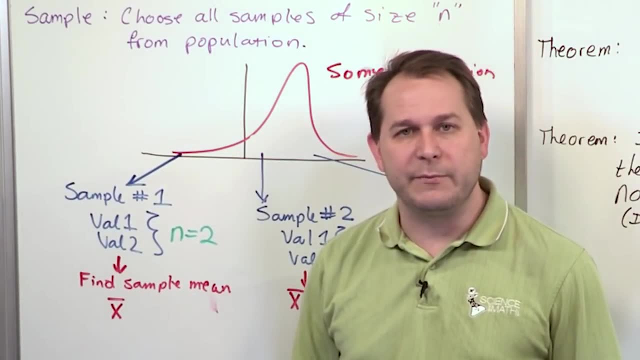 actually is normal, which we've already said is the lion's share of the cases in the real world- then the distribution of these sample means right. the distribution of the sample means is going to look normal. It'll have a normal distribution. 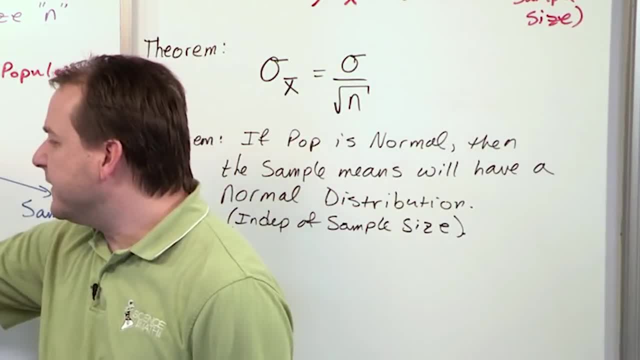 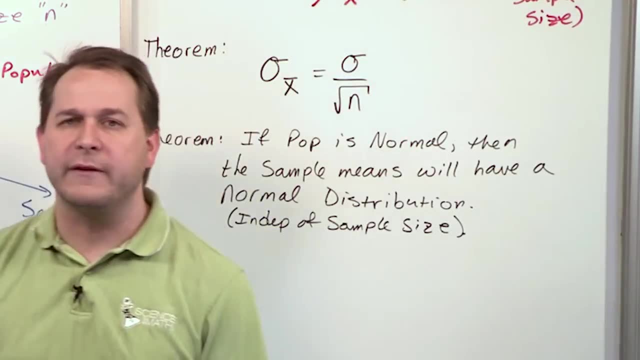 In other words, obviously if I sample this guy and get an average value, I'm going to get a slightly different value from the next set of samples and a slightly different value from the next set of samples. But if I were to look at the frequency of when these different means? 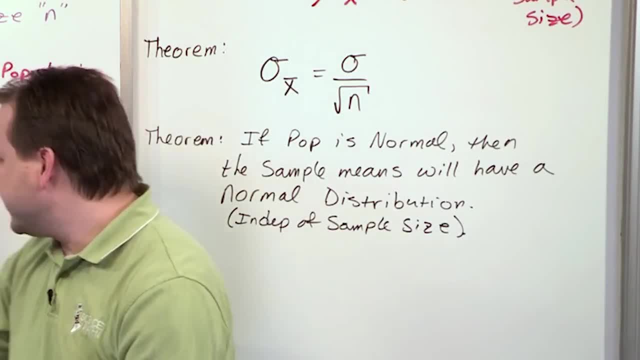 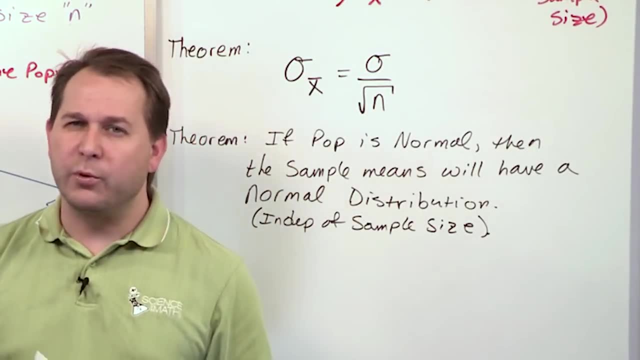 pop up. I'm going to find out that the peak of this guy, the relative frequency, the peak of my sample means that I get- is going to look like a normal distribution. That's very important for you to know because we know how to work with normal distributions. We've spent a lot of time 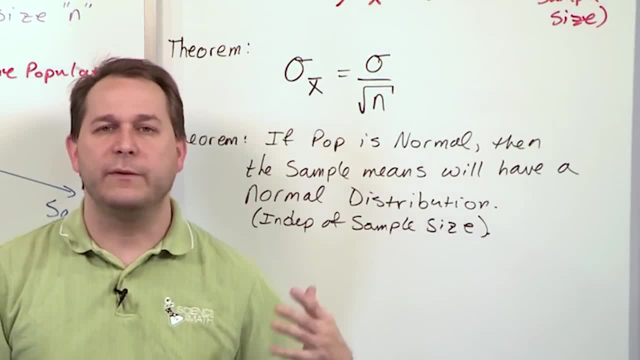 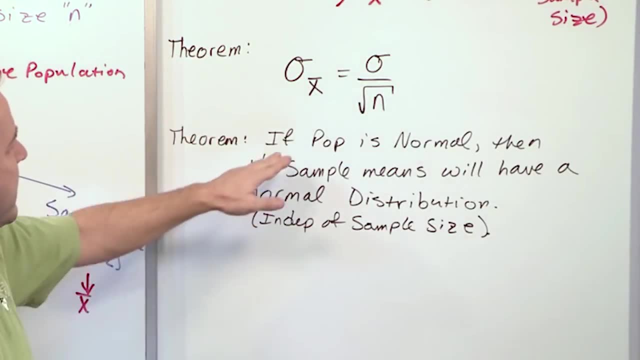 using the Z chart table: normal distributions. We've done a lot of work with learning how to solve problems when things look normal. Now we're saying if the population's normal, then the sample means when you look at the sample means they're going to look normal too. Now that's. 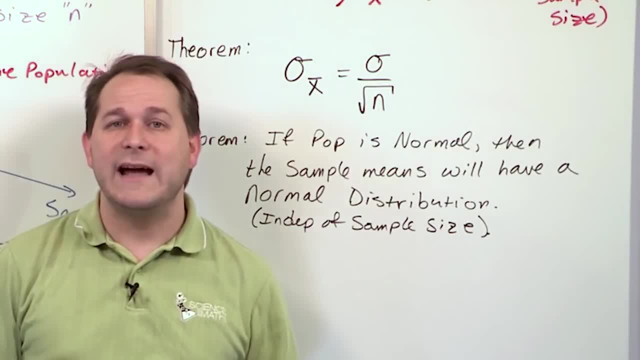 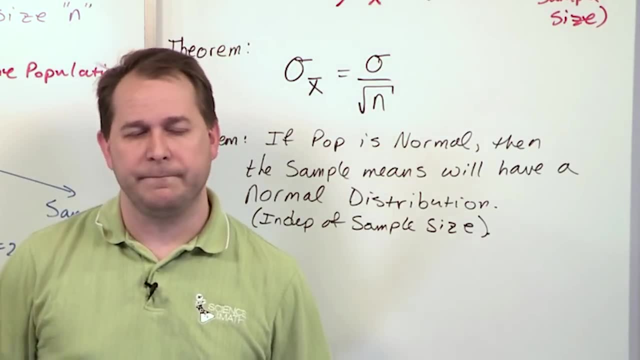 pretty darn useful and we're going to solve some problems where you can see how to really use that, But it shouldn't be mind-blowing that if the parent population is normal, then the sample means will also look normal. Okay, Now here's the part that probably will be the most important. 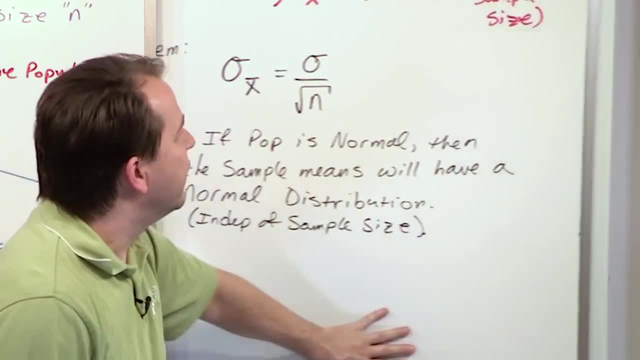 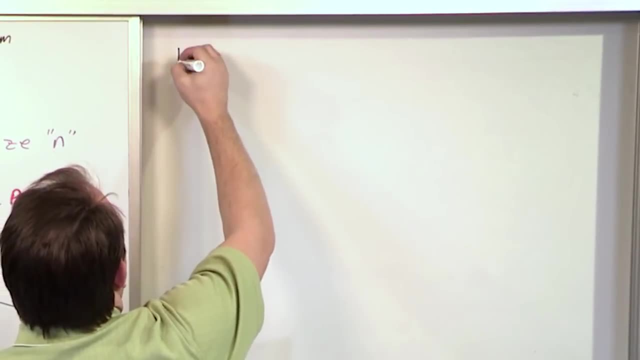 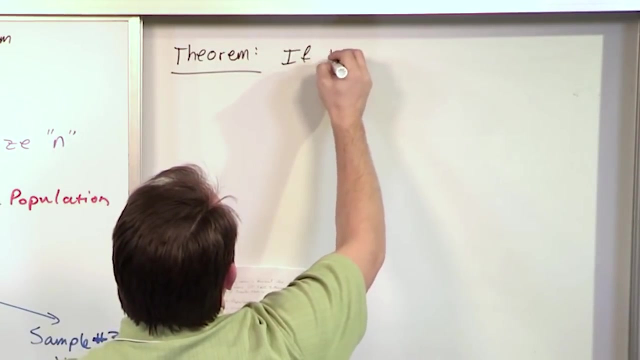 because it will blow your mind. and if it doesn't blow your mind then I'm not doing my job right. So I want to give this guy his own little part of the board here. So the last part of the central limit theorem is the following: If the population is not- I'm going to underline that- 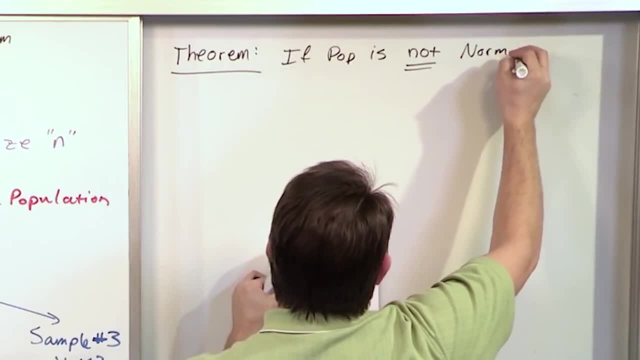 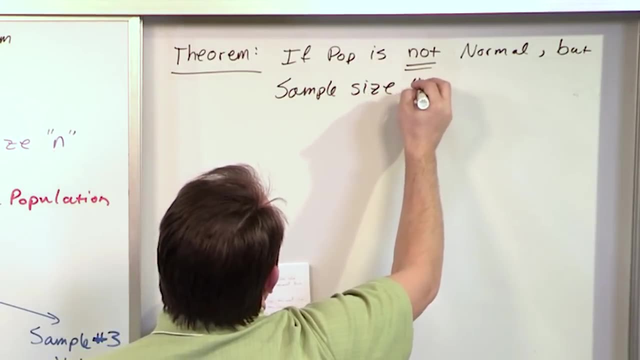 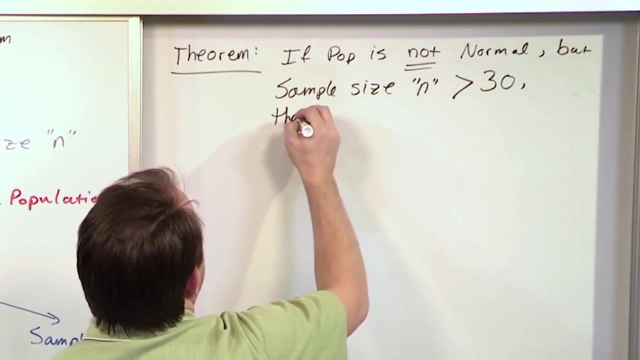 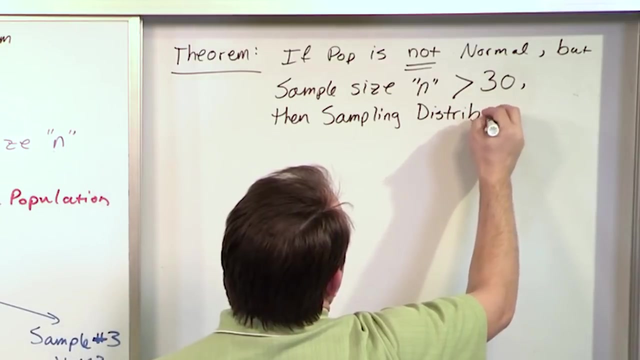 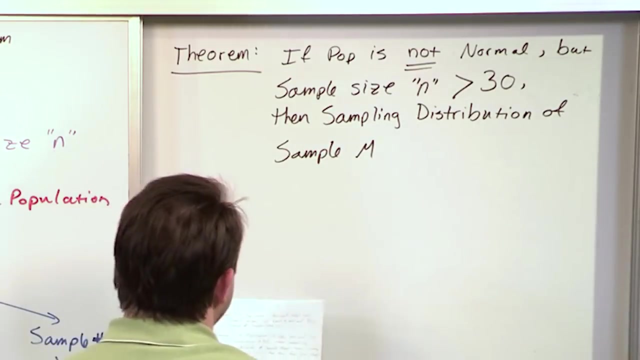 two times because it's important, not normal, but the sample size is not normal, then the population which is called n is greater than 30.. Okay, Then this is what we call the sampling distribution of sample means, which is just the data we've collected after we found the sample. 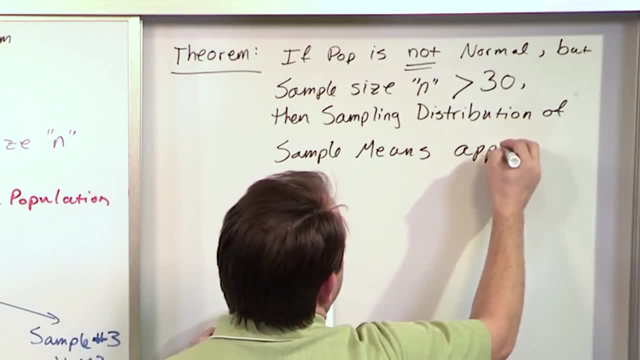 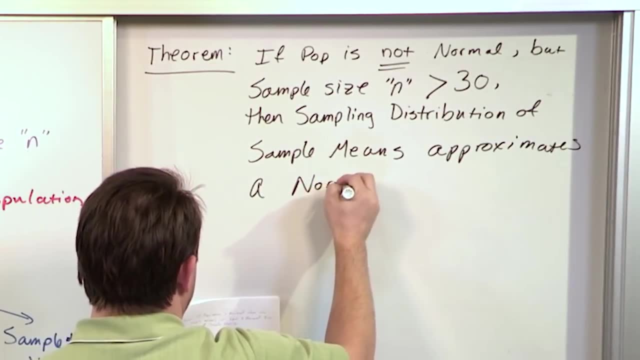 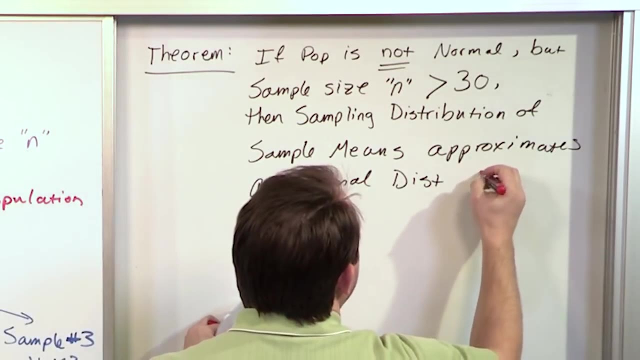 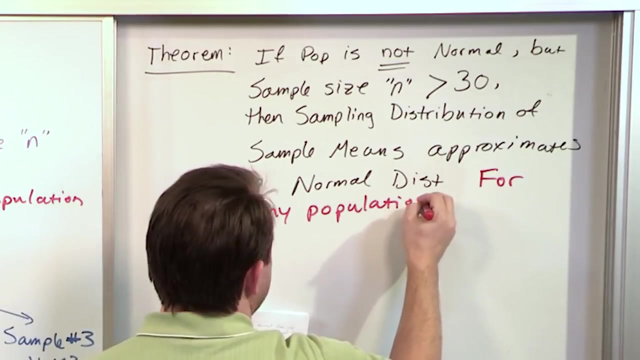 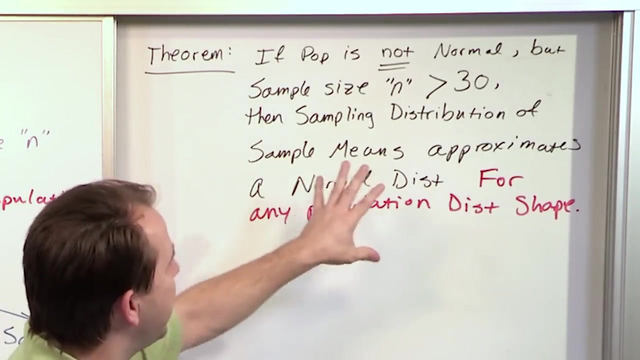 means approximates. Guess what it approximates A normal distribution And I'm going to put in red for any population distribution shape. I know that the significance of these words don't make a lot of sense until we start solving problems and things, but it's truly remarkable and this is what I'm going to. 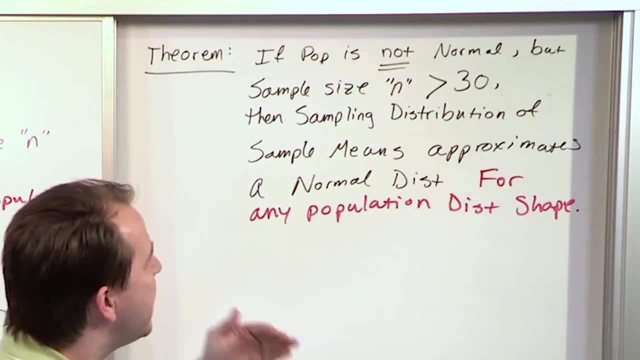 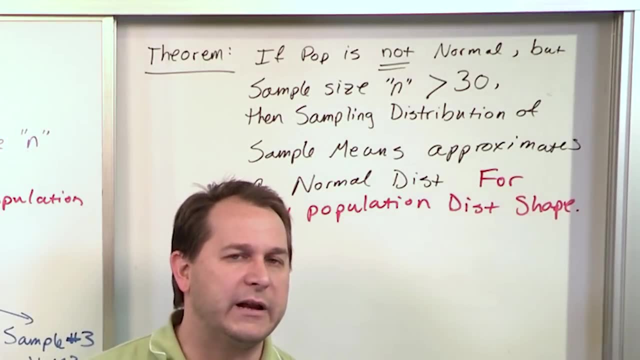 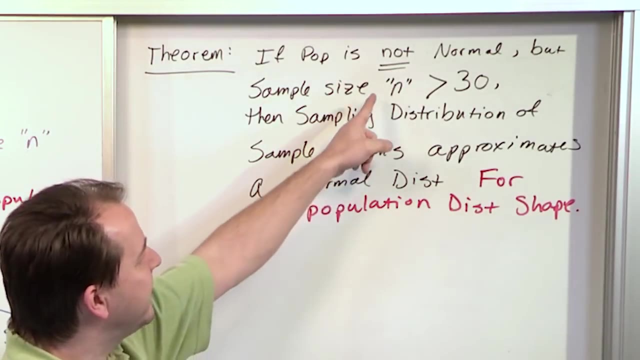 talk about what is really so useful about the central limit theorem. If I choose to study a population, right, if I choose to study a population, even if the parent population is not normal, let's say it's skewed or uniform or squiggly or just something really weird. if I choose my sample, 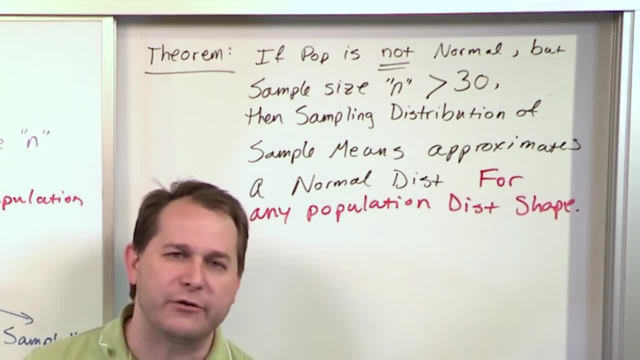 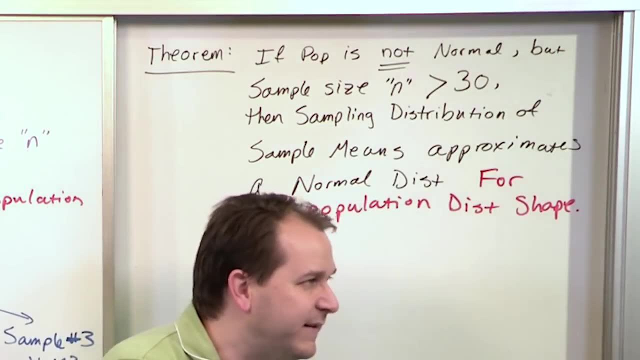 size in large. large meaning greater than 30,. they've calculated the value. 30 is the magic number. alright, so just remember that If you choose a sample size greater than 30, and I sample this 30 people and then this 30 people- 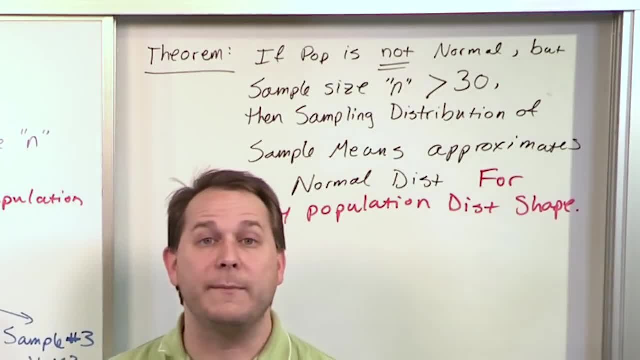 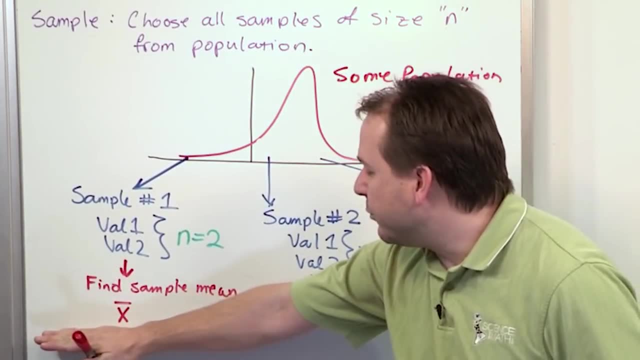 And then this 30 people, And then this 30 people And I do it for the whole population. I get all my data right and then I look at the sample. sampling, distribution of sample means. that means here's sample mean number one, here's sample. 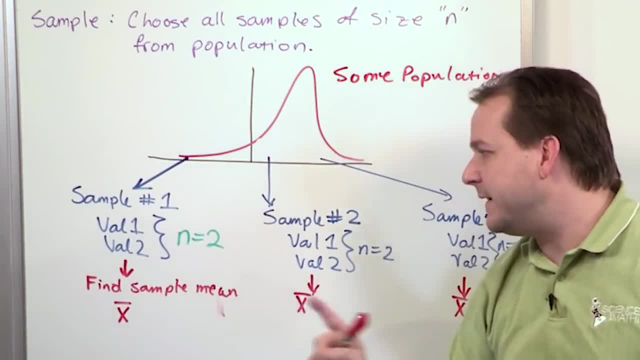 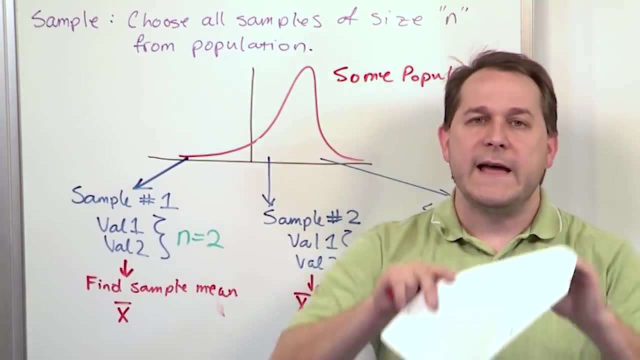 mean number two. sample mean number three. I'm doing it for the whole population, but in this case I'm doing 30 values each time. 30 values each time. I'm getting a sampling distribution of sample means And then I plot that on a histogram. it's going to look normal, Even if the original population looks. 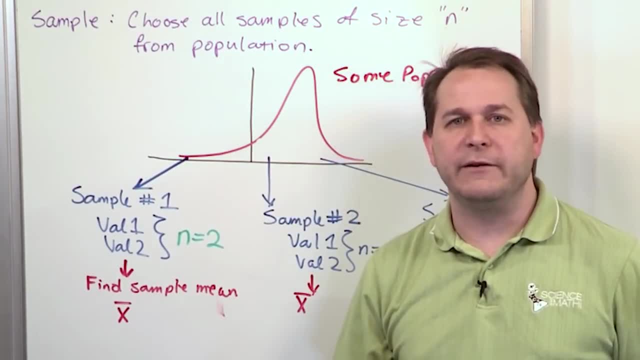 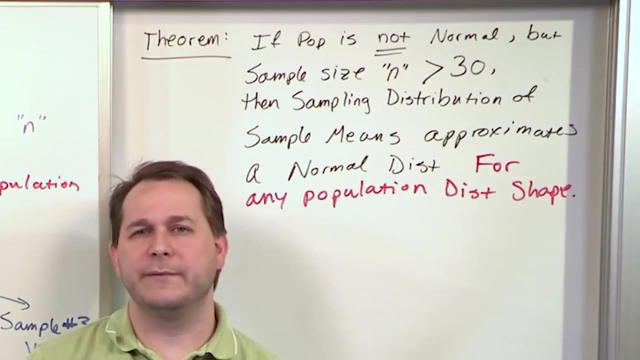 weird and skewed or non-symmetric or something else. It's truly. it's truly impressive. it's truly amazing. and you might ask: why do I care about that? you built up the central limit theorem so much. why do I care? The point is, I don't need to know what my parent population looks like. I don't need. 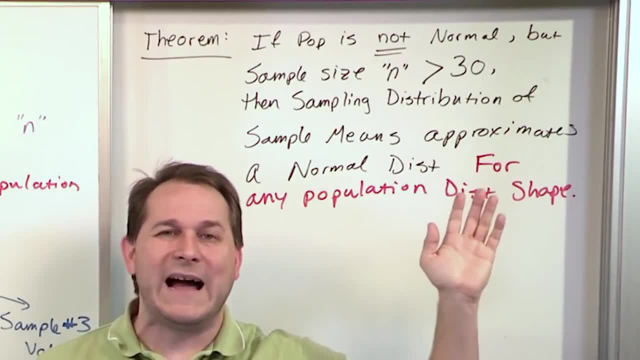 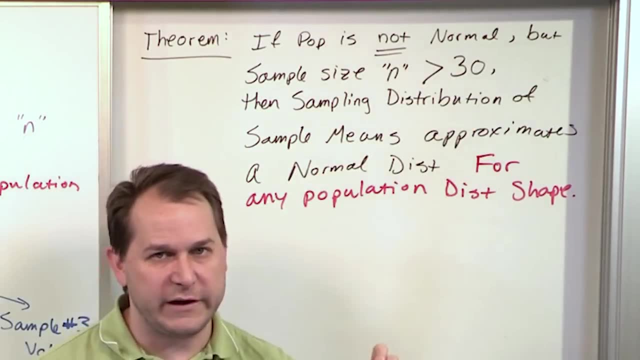 to know what the population of a North American adult male's IQ is. I don't need to know if it's skewed, symmetric, uniform, normal, it doesn't matter, As long as I sample it with a greater than 30, then the 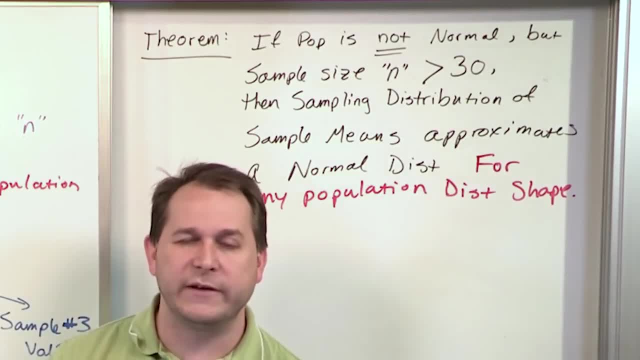 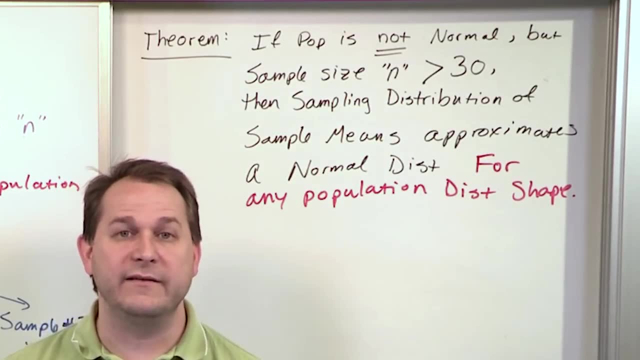 sampling. distribution of sample means that I get is going to look normal, And I like that because I know how to deal with normal distributions. I have an entire chart in the back of my statistics book that deals with normal distributions. So by just selecting the sample size greater than 30, it then allows me to solve. 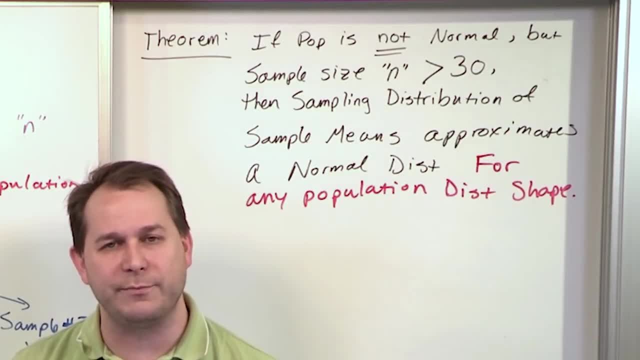 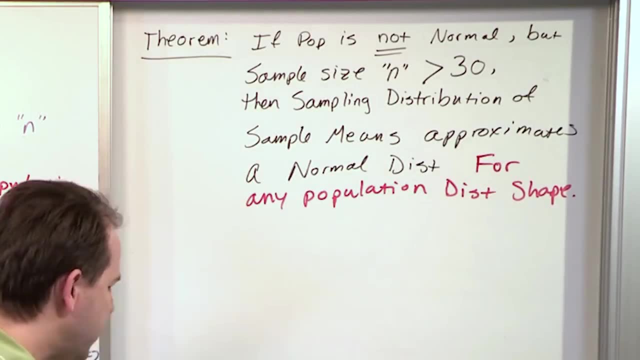 tons of problems because I know how to work with normal distributions. I can use those charts in the back of the book to solve lots of really, really practical problems because of that. So let me draw one little graphic to wrap this up and show you what I mean. 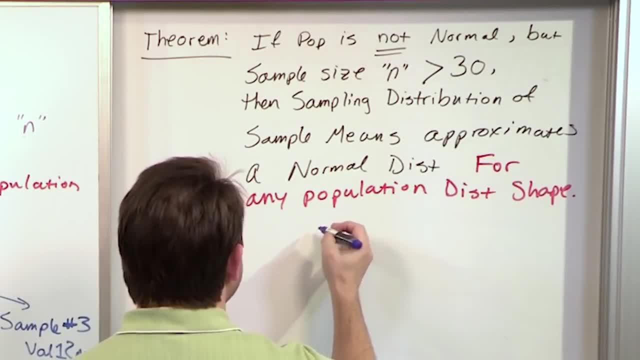 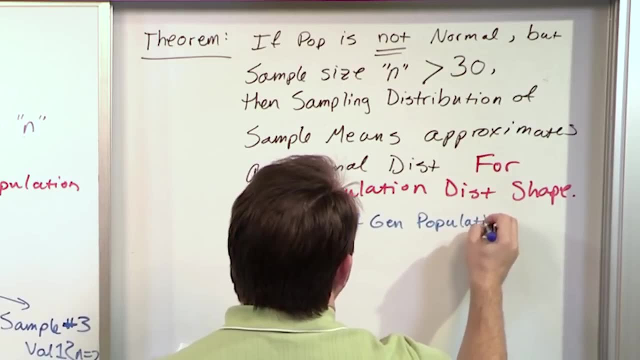 This is what I'm talking about. Let's say that the IQ of the general population, let's say of the world, is something like a normal curve. That's kind of what I would expect, to be honest with you. that's what. 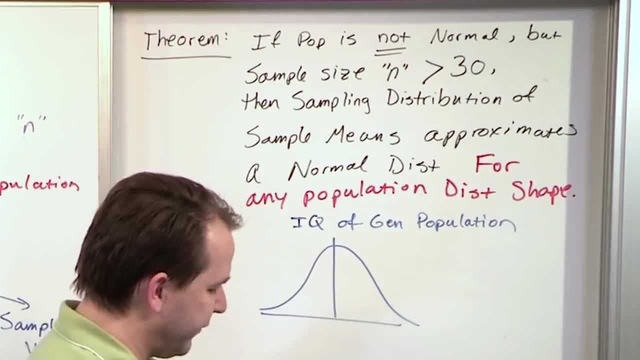 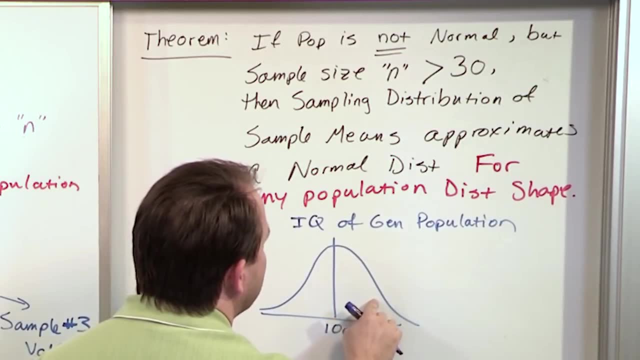 the IQ is supposed to be. They're supposed to design the test so the average person has like 100 IQ. So that's right in the center. Now, as you start getting higher than 100, less and less and less people have an IQ that high. 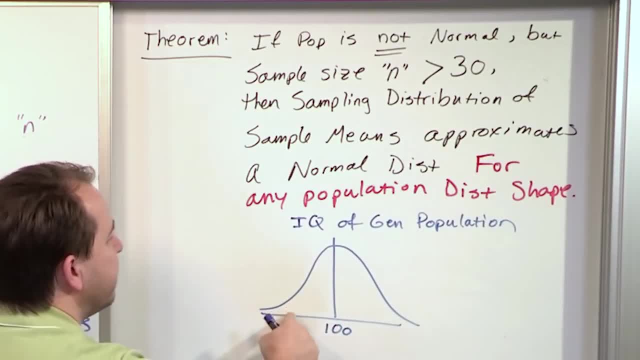 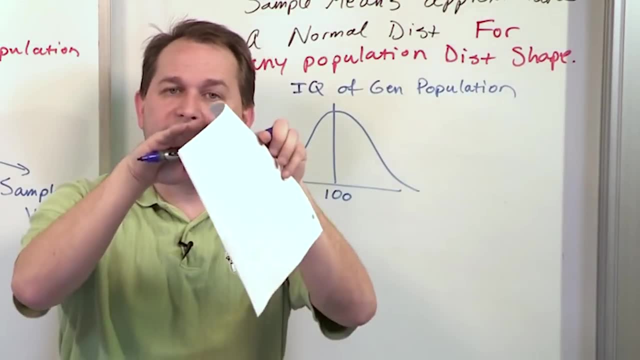 And below 100, less and less and less people have an IQ lower than 100.. And I haven't drawn it perfectly. It's supposed to be exactly symmetrical. The test is supposed to be designed to be perfect so that it's measuring. 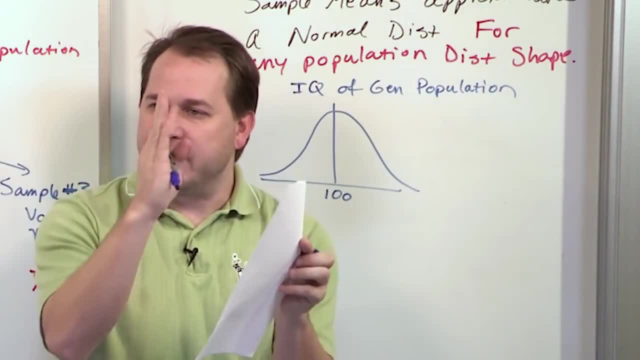 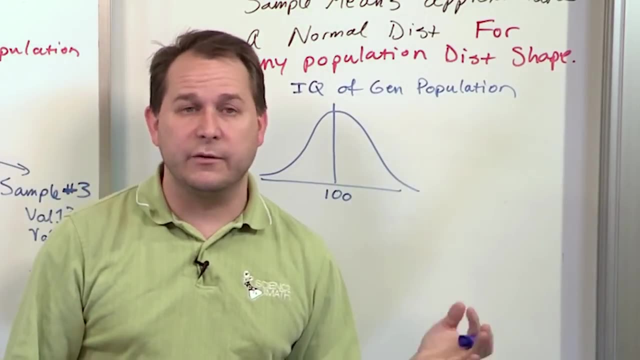 the average intelligence of human brain And you have some people on the left and some people on the right. The Albert Einsteins are way over here- And then, unfortunately, you have some people who are deficient and they're way over here. Some people score not as great on those types of tests, But this would be the IQ of a general population. 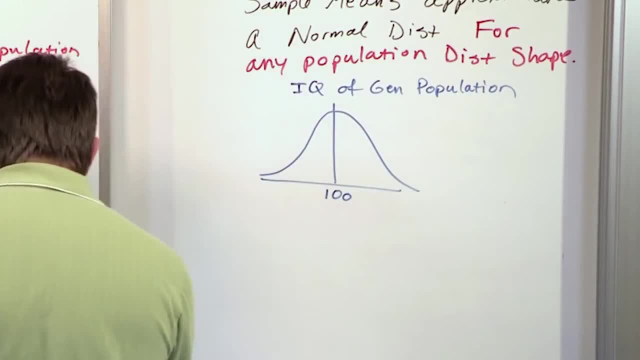 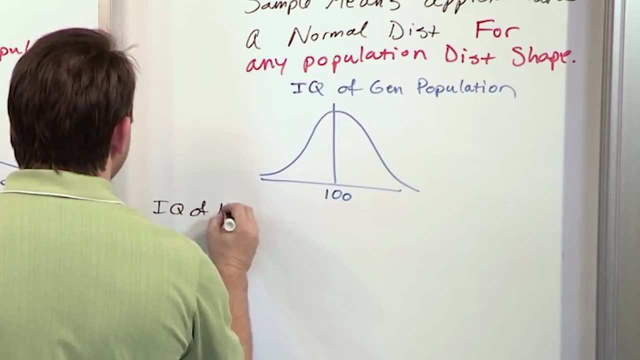 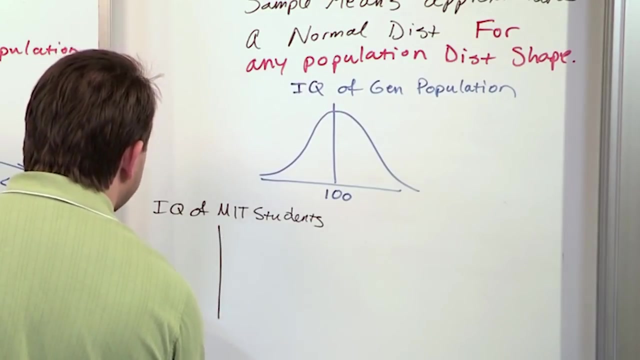 Now let's pretend that we're not studying a general population anymore. Let's go and study the IQ of MIT students. I'm choosing MIT because most people would agree that it's one of the best universities in the United States. But there's lots of them. It could be Stanford, It could be tons of other universities. 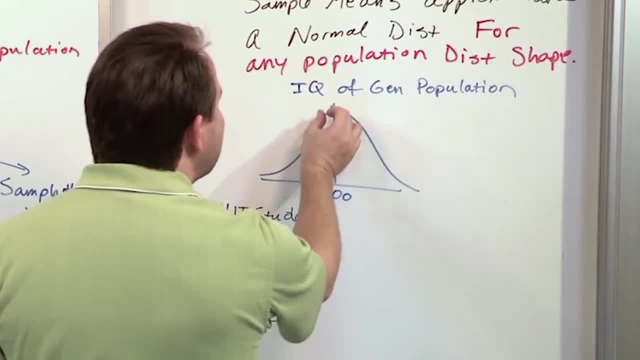 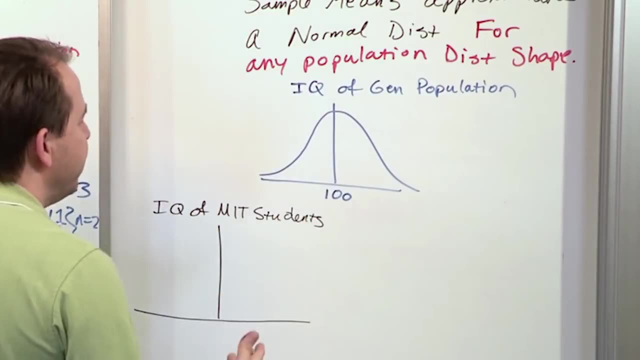 Now we would expect that the IQ of MIT students would not be perfectly symmetrical like this. We would expect that the average value of a student at MIT, the average student IQ, is not going to be 100. Because when they select those students, they're throwing out a lot of the lower scoring people. They just have to. 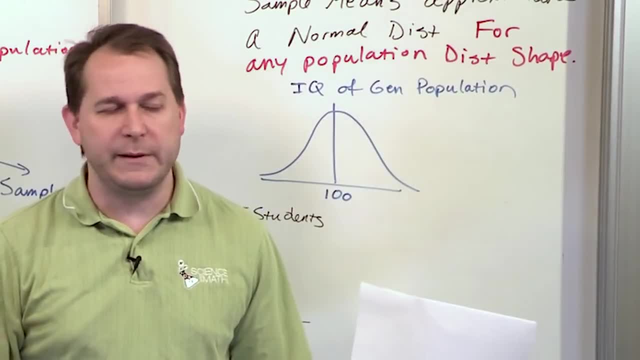 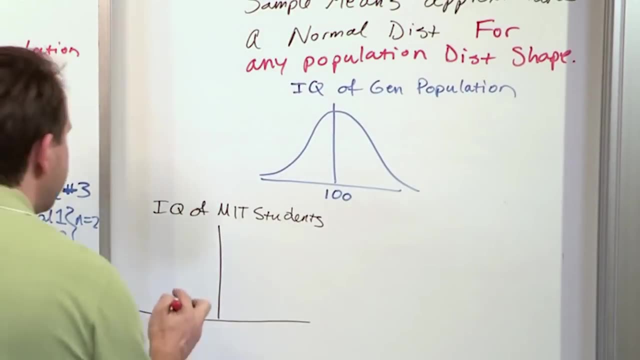 So when they test those guys and they pull them in, they're generally pulling the people that have scored higher. So we would expect this distribution not to look like this one here. I don't know what it looks like, I'm just making this up, But it might look something like this: It might go and have a very sharp peak and then a very sharp drop off. 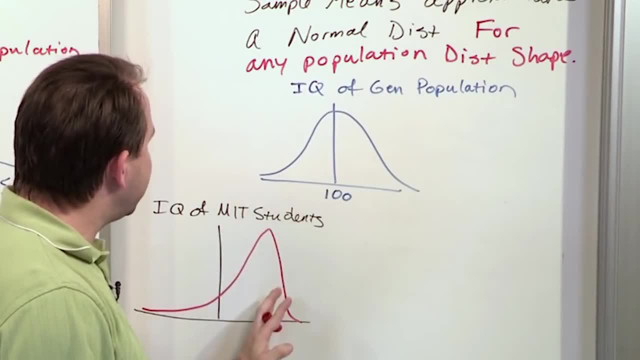 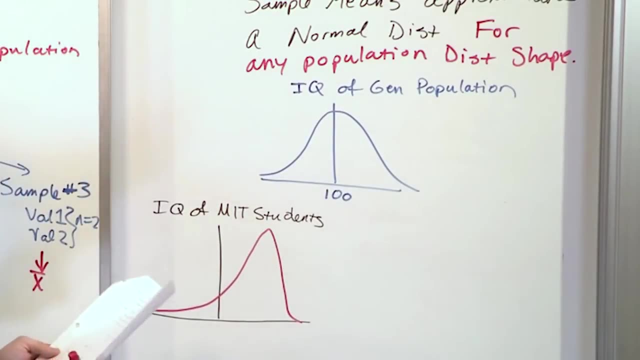 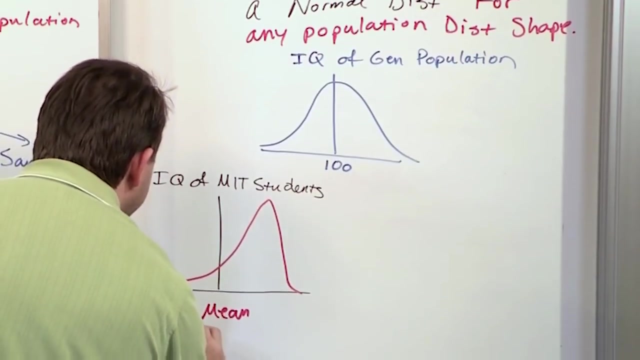 So a lot more students may be up around 100.. You may be up around 110 or 120, with a very sharp drop off here And you can definitely see where the vast majority of your students are. And then we can say, for instance, say the mean mu is a mean IQ of 125. 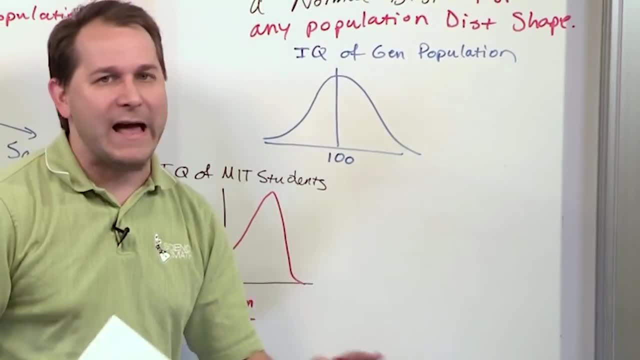 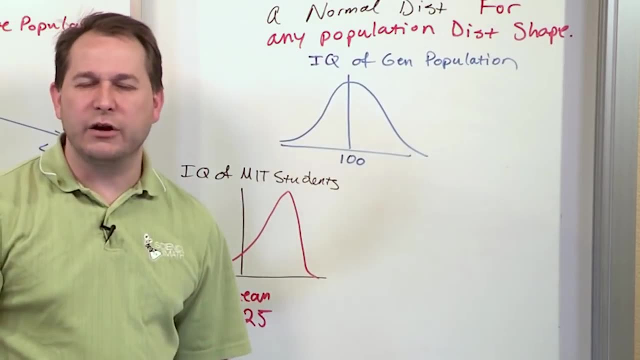 I'm just making this up. I have no idea, So please don't take this information as fact, because it's not fact. But they'll say: the IQ of the general population is 100, the average IQ, The average IQ of a student at MIT, is 125. 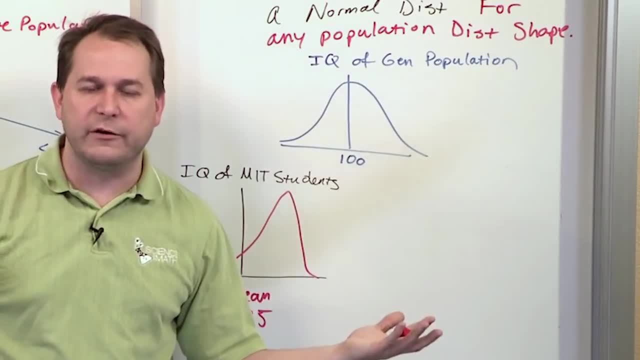 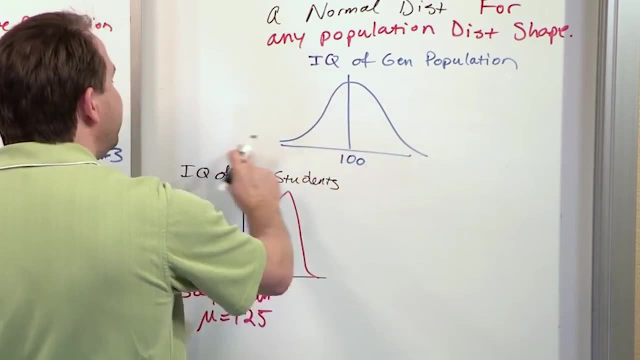 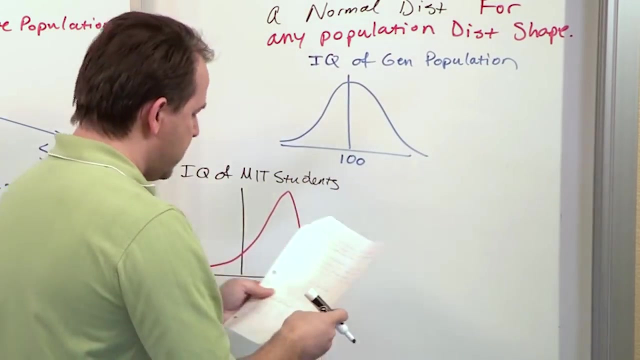 Of course, this is shifted higher because of what we just talked about. Now, what it's saying, what the central limit theorem is saying, is: if I choose the MIT students as my population, so I'm no longer studying the general population, I'm only studying the IQ of MIT students. at this point, 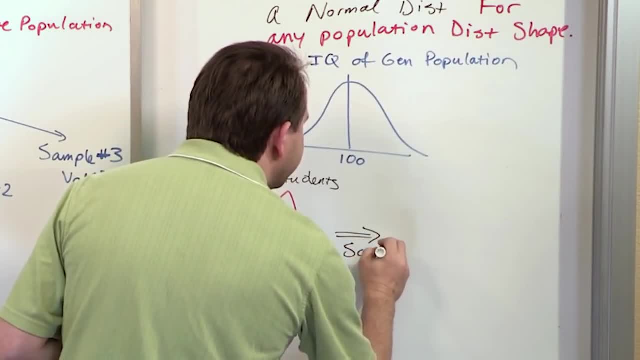 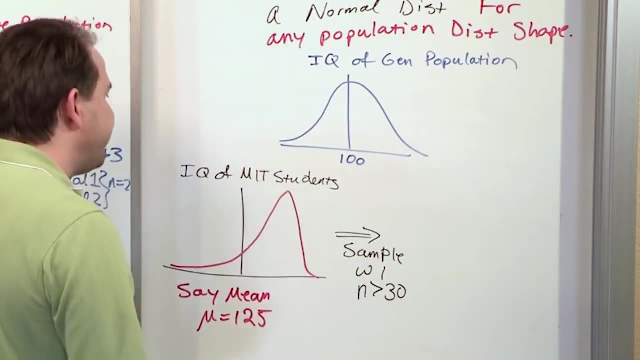 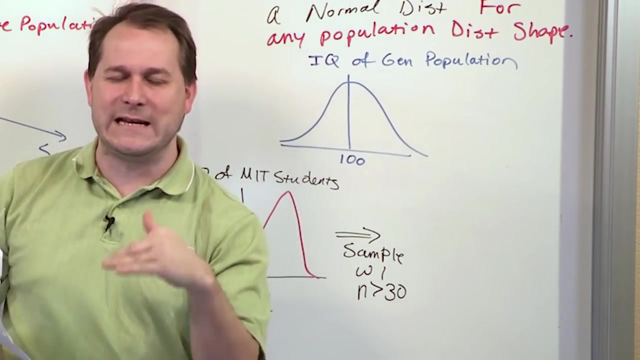 If I then sample these students with a sample size greater than 30, so I take a sample of 30 MIT students and another sample of 30 MIT students and another sample of 30 MIT students, And every time I do it I calculate a sample mean. 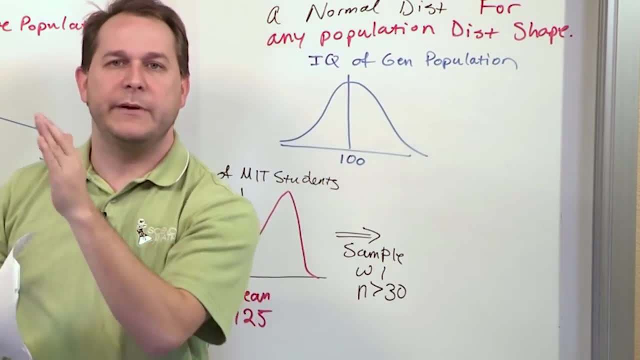 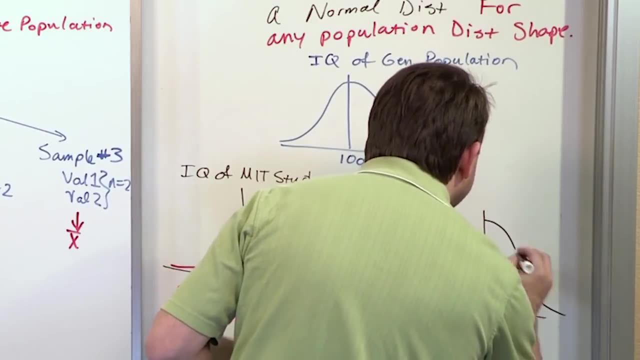 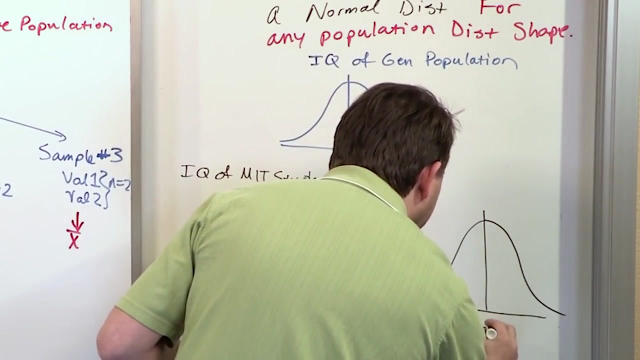 So I'm going to get a sample mean for sample number one, another sample mean, another sample mean. another sample mean Then what I'm going to get when I construct that is a normal distribution. The average peak of this normal distribution will be 125. 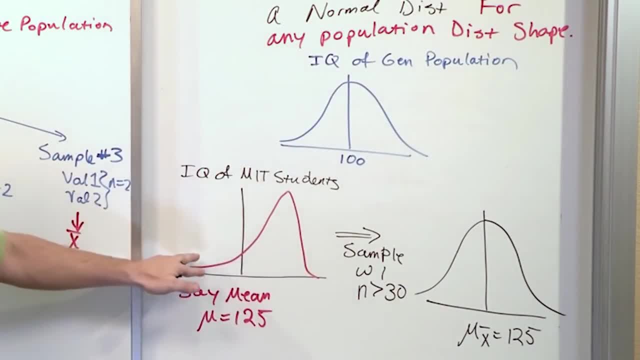 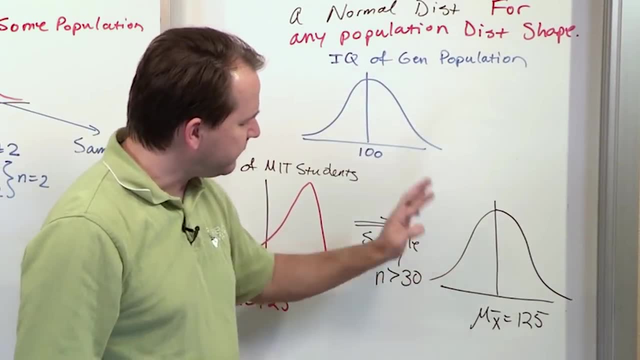 Even though the original guy- the original guy- the average peak of this distribution will be 125.. The original curve looks weird and skewed in a weird way. When I do the sampling distribution of sample means I'm going to find that the peak of this normal distribution is right at 125. 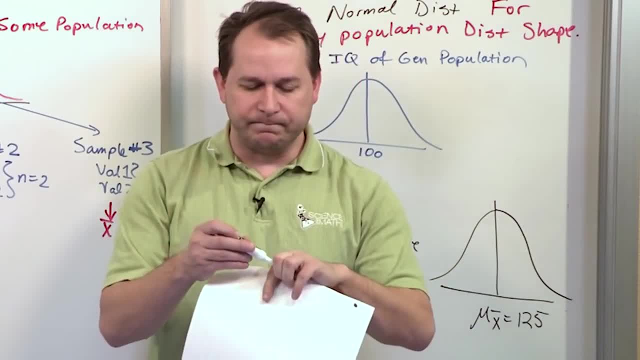 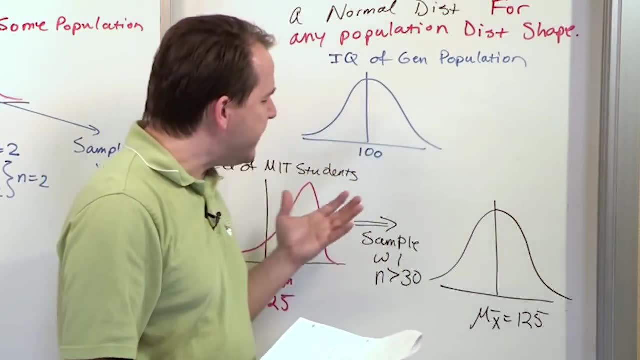 and it normally falls off on both sides. And the reason that that's useful is because if I'm going to study MIT students and I'm going to solve a problem, and we're going to solve lots of problems in the next section- if you choose your sample size large enough, 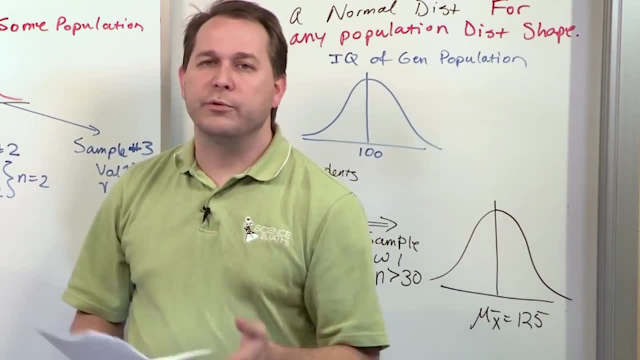 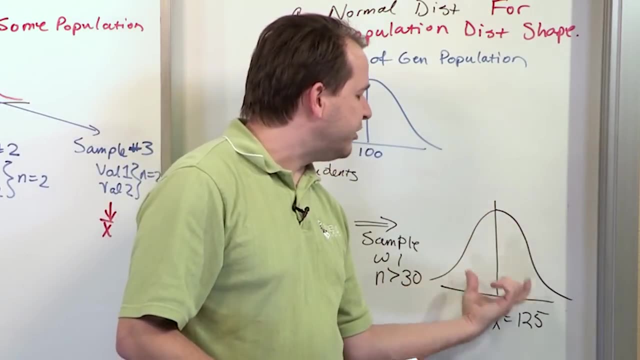 then you know that the answer you're going to get is always going to look normal. So I'm going to use the normal distribution Z tables in the back of any statistics books to calculate lots of useful information. And this normal distribution comes about no matter what the shape of this curve is. 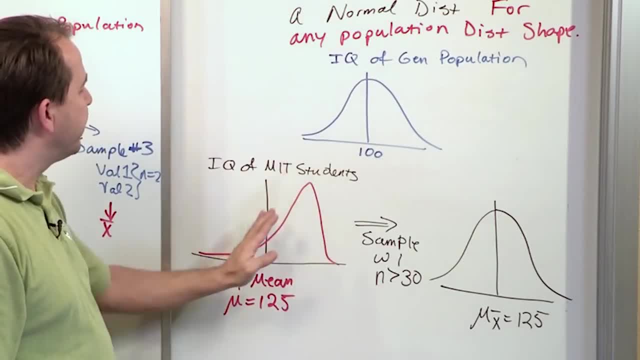 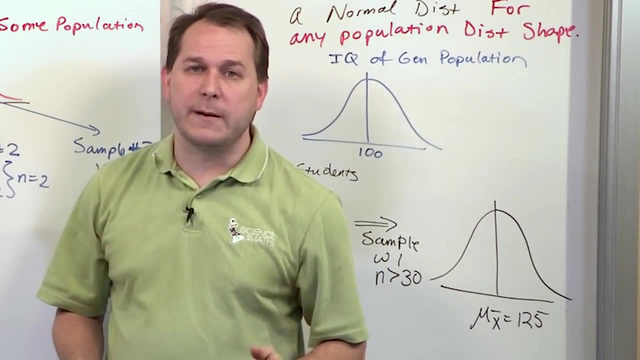 This could be uniform. This could have some weird squiggly lines. Who knows what the distribution is. It's irrelevant If I sample with a greater than 30 and I take lots and lots and lots and lots of samples from my population. 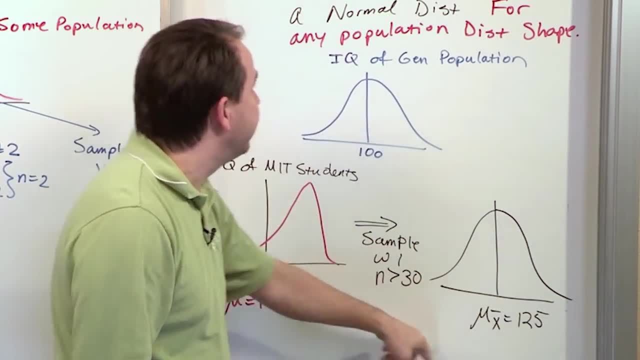 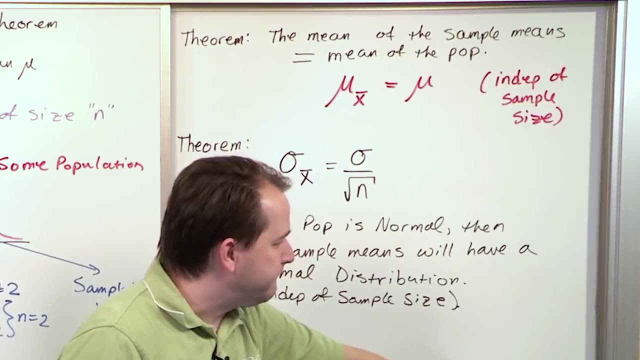 then what I'm going to arrive at is an average value of 125, because, don't forget, the mean of the sample means is always going to be equal to the population mean, right? So that's why it's centered there and it's going to look normal. 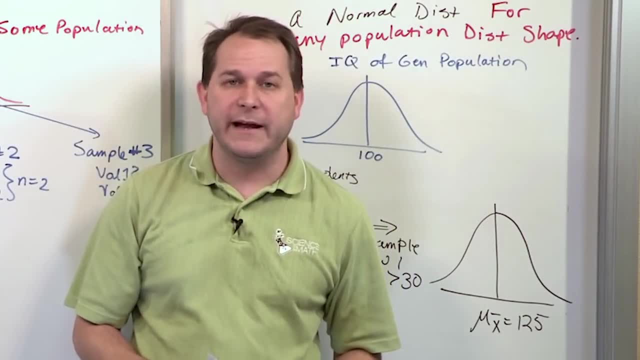 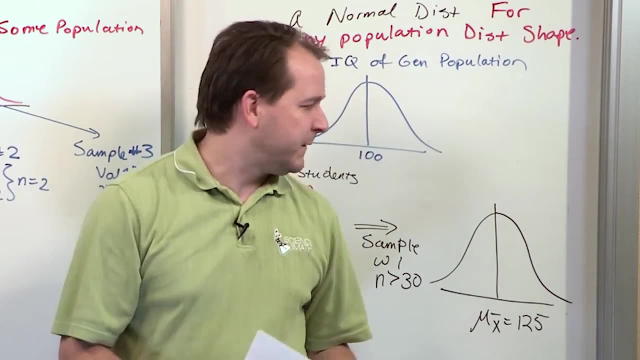 I'm not proving that to you. I'm not going to do that kind of proof because it's very complicated proof and it's beyond the scope of what I want to teach you here. What we want to do is learn how to use the central limit theorem to solve problems. to solve problems. 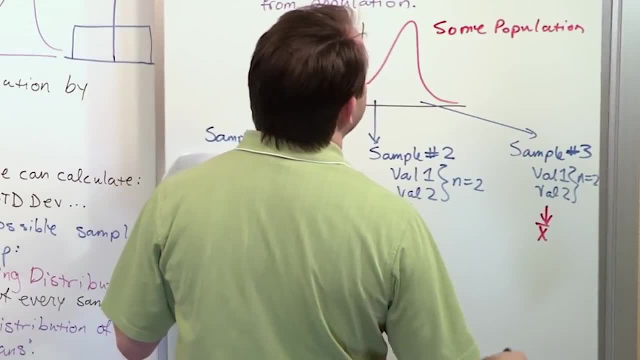 All right. so I want to do a quick recap of everything because I don't plan to revisit this stuff again. What we're going to do is go work. a lot of problems, but I want you to have a nice mental image. 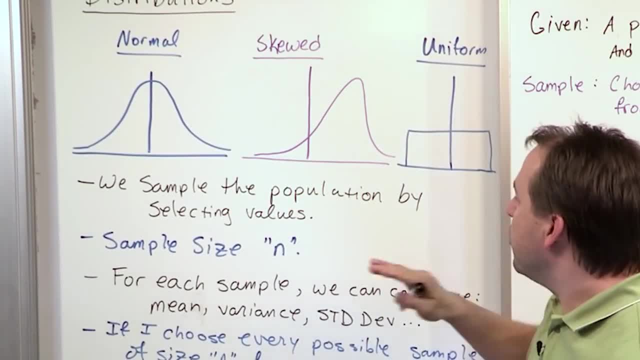 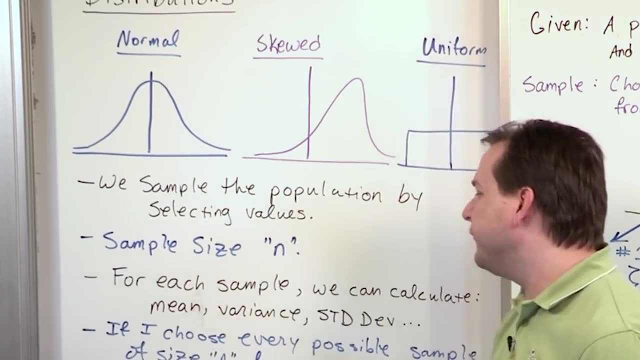 So what we're saying is: distributions can be any shape and size, all right. We sample the population by selecting values, The sample size, we call it n. We can calculate mean variance, standard deviation. We can also calculate something called proportion- we'll talk about later- for every sample that we have. 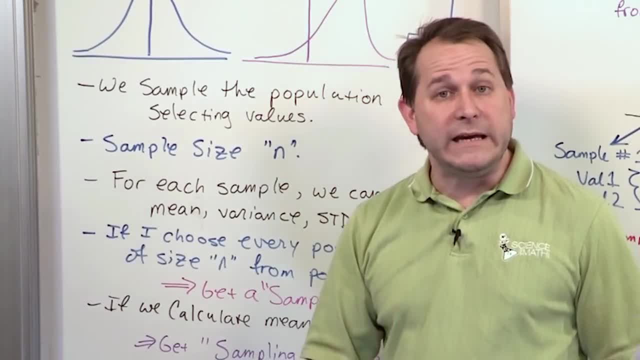 And then I get a sampling distribution as a result of that. Now, when I'm talking about means- which is a lot of time, what I'm trying to do- I call it a sampling distribution of sample means. That's what I'm talking about. 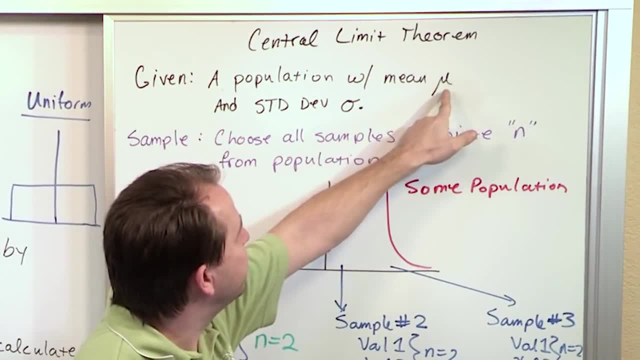 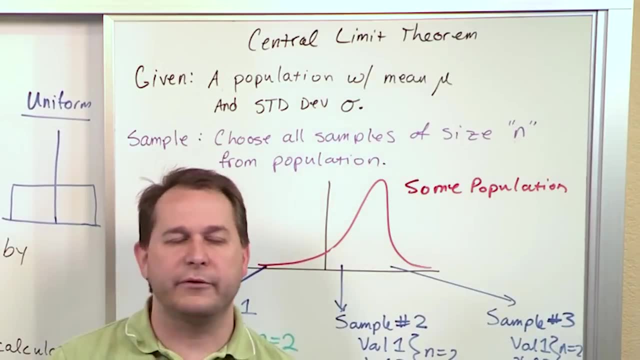 So for the central limit theorem, we're always going to have some population with a population mean and a population standard deviation. I choose all the samples from the population. I keep going until all the samples are exhausted. I choose a sample size of n from the population. 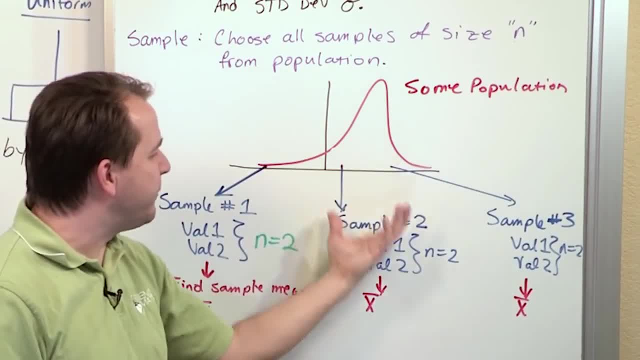 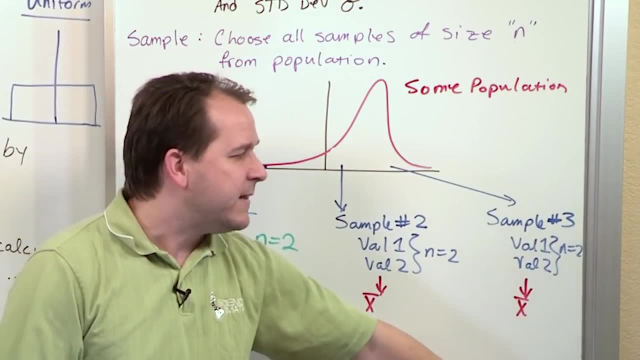 I don't know what the shape of the population is, but I collect sample one, sample two, sample three and so on. keep going until the population is exhausted and I can calculate these sample means along the way. That's going to give me a sampling distribution of sample means. 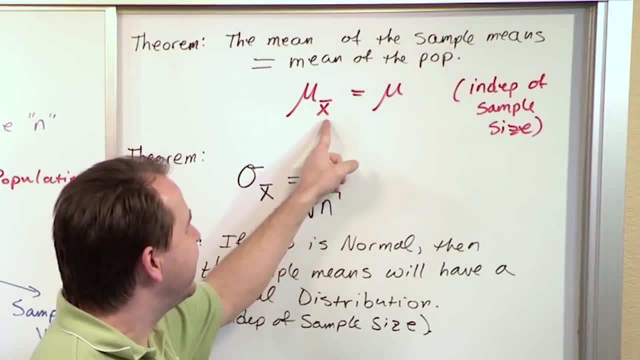 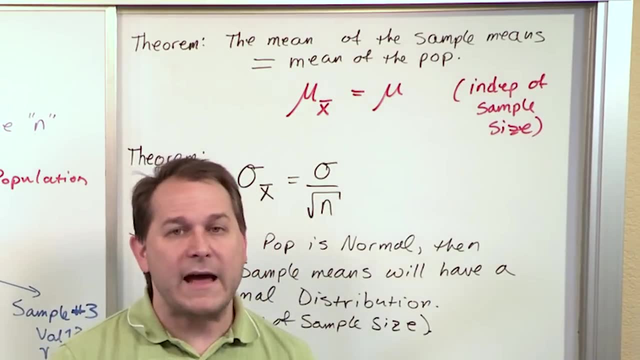 Central limit theorem says that if I take all of those sample means and I average them together, the answer I'm going to get is going to be equal to the population mean It doesn't matter what the sample size is and it doesn't matter what the shape of the original distribution is either. 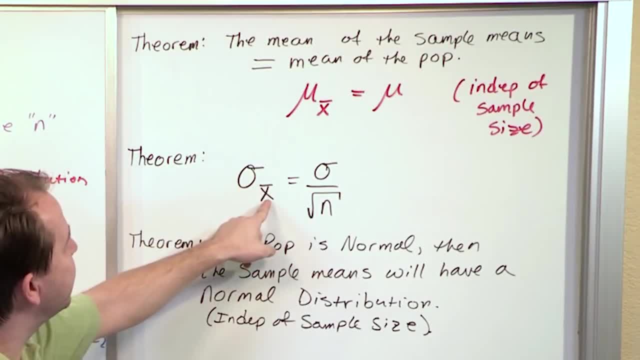 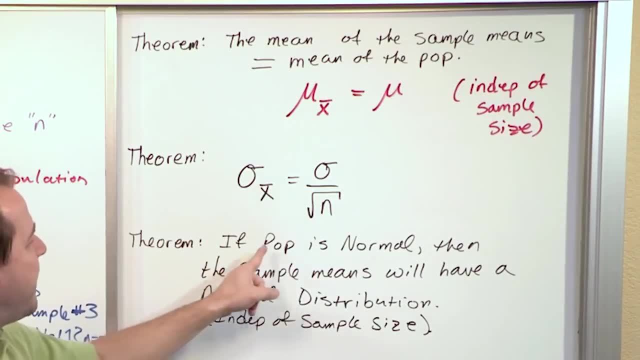 The standard deviation of the sample means can be related to the standard deviation of the population, So that's important as well. If the population happens to be normal, then the sample means will always have a normal distribution. It doesn't matter what the sample size is in that case. 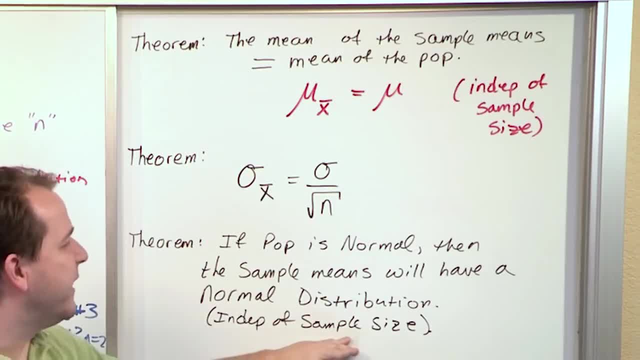 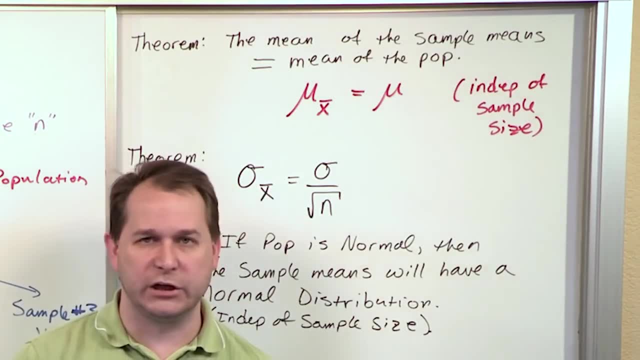 Notice how I said it. It doesn't matter what the sample size is. If the parent distribution is normal, then I don't care what the sample size is. My distribution of sample means is always going to look normal. But in the case that the parent population is actually not normal, 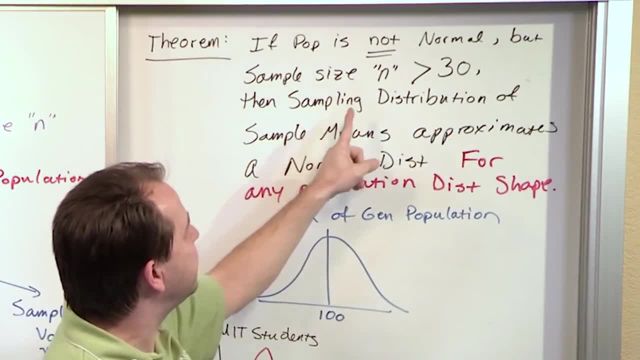 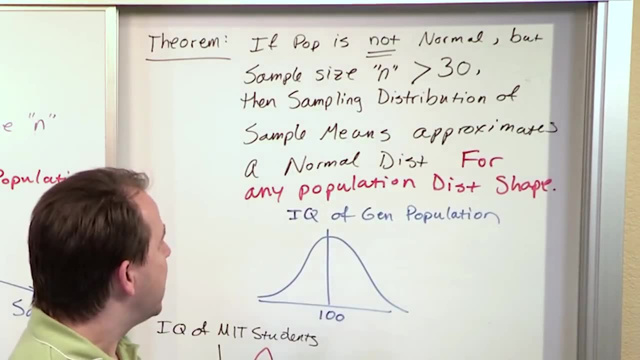 if I choose a sample size greater than 30, then the sampling distribution of sample means looks approximately normal anyway, And there's lots of math proving that. but that's true, And it's true for any population, And it's true for any population. 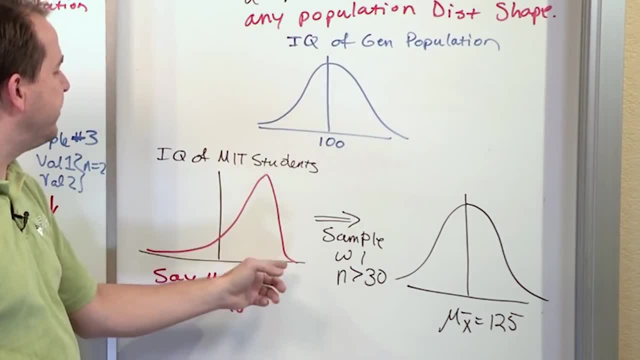 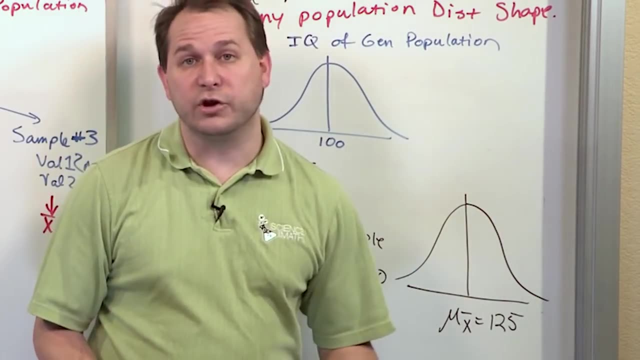 But it's true for any population. So this is a very important part of the calculation distribution shape. So we use the example of studying MIT students. We have a skewed distribution If we take lots and lots and lots of samples and find their sample means. 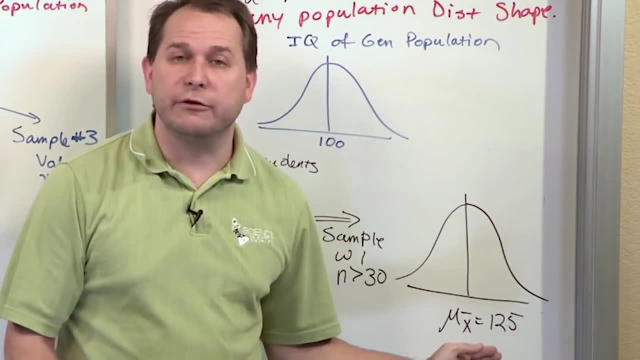 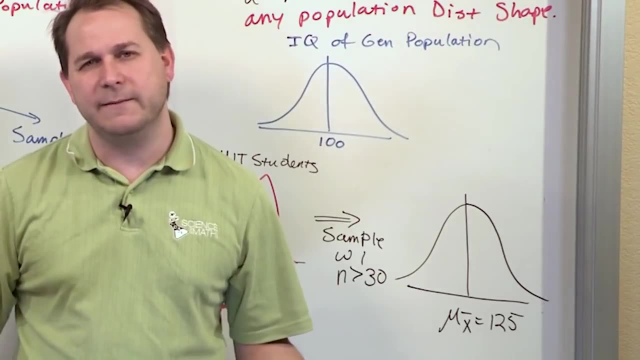 and plot them. on a probability distribution like this, it's going to look normal where the majority of what I'm going to be calculating for the sample means, will end up falling right around 125, because when you think about it, it's pretty close to the average IQ of MIT students. 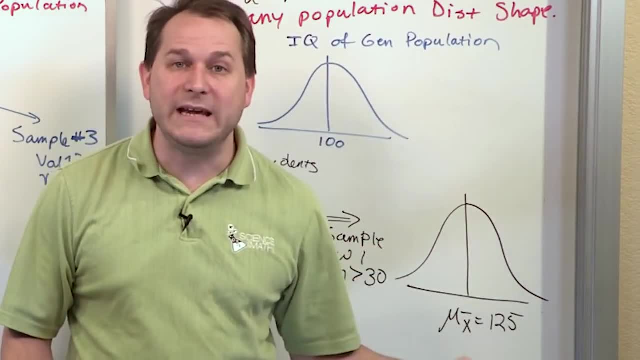 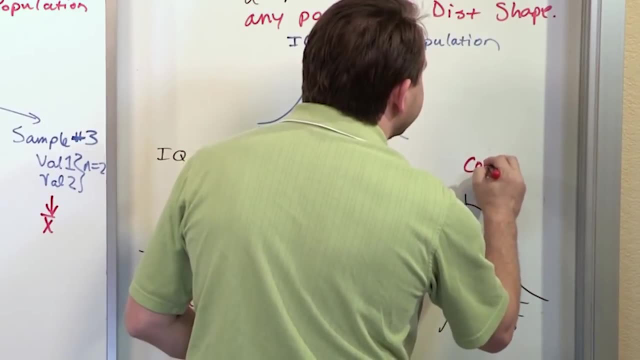 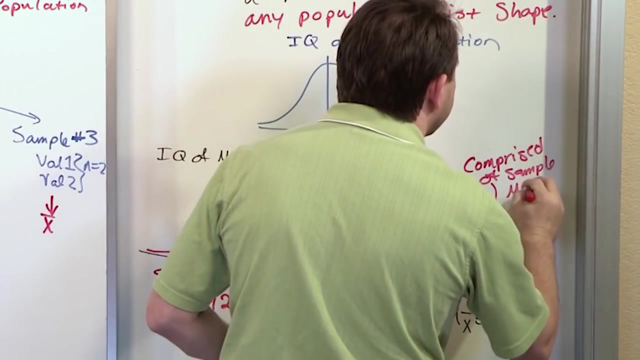 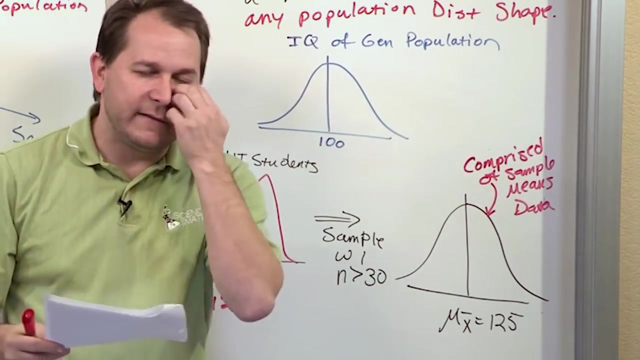 But of course I could get some calculations of the sample mean lower or higher than that. This curve, this entire curve, is comprised of sample means data, So it's the data I get from the sample means is what comprises that, And that is the punchline for central limit theorem. 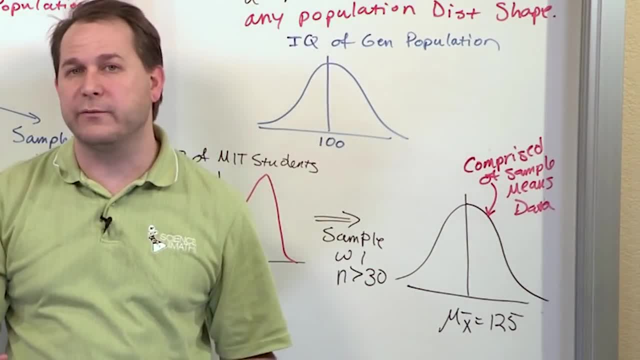 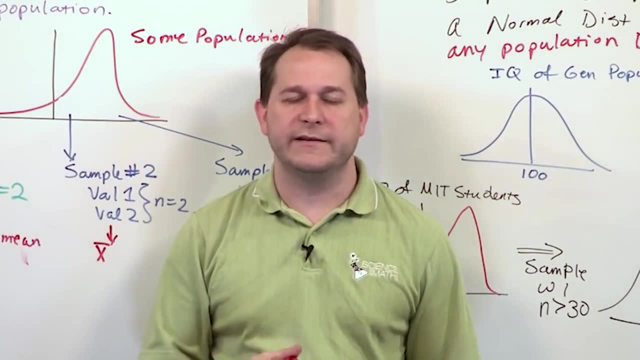 I don't fully expect you to understand how important or useful it is right now, because we have to solve some problems. So I'm going to stop here and I'm going to let you absorb that. mull it over. Follow me on to the next section. 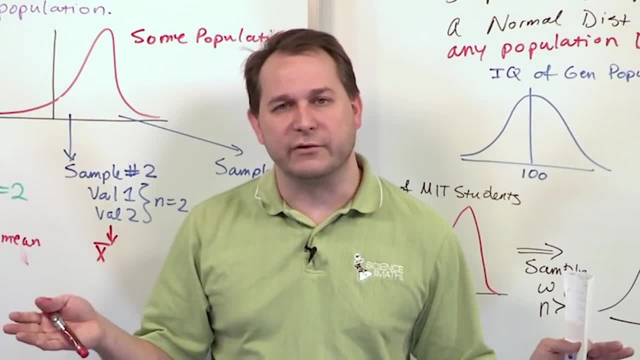 I promise you we're going to get into some real problems. There's a lot of overhead with the central limit theorem. I have to explain it, And if I don't then you're just not going to understand what we're doing. So I've tried to do my best to explain what it is. 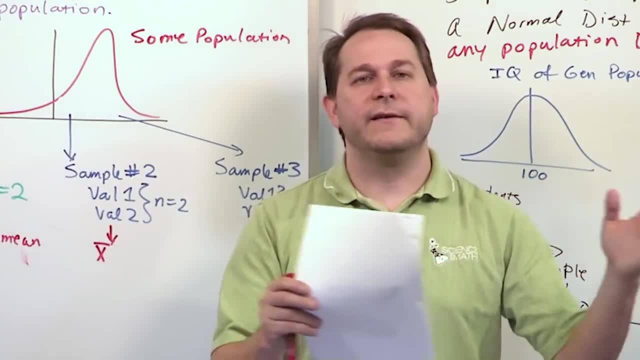 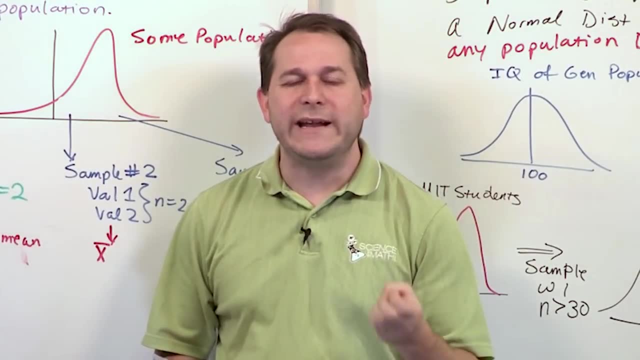 I've tried to explain the difference between a sample size and a sampling distribution and kind of get these terms comfortable in your brain. Now, when we go to the next section and you read a problem, you'll know exactly what it's asking, And so let's do that now. 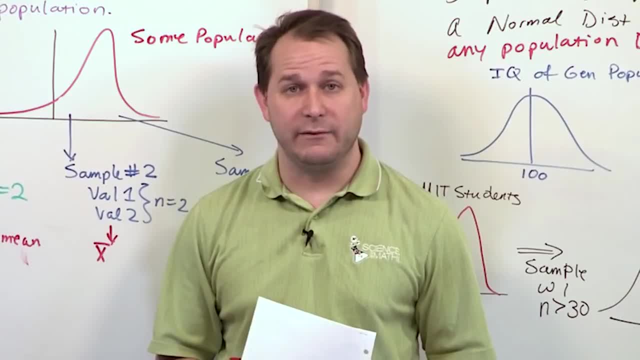 Let's go on to the next section, where we'll solve some problems with the central limit theorem.